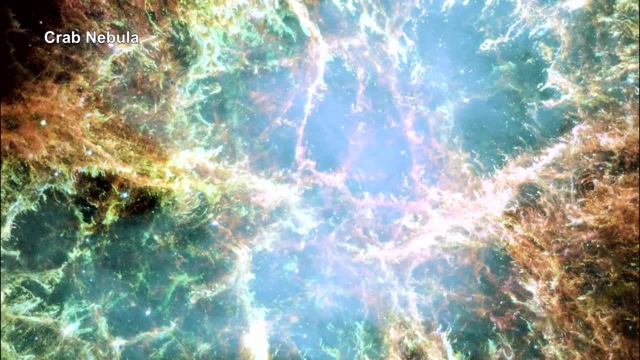 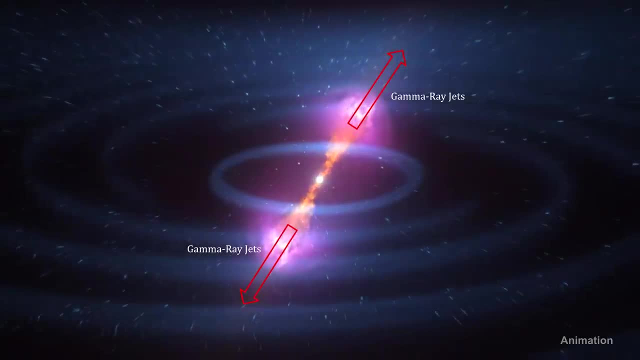 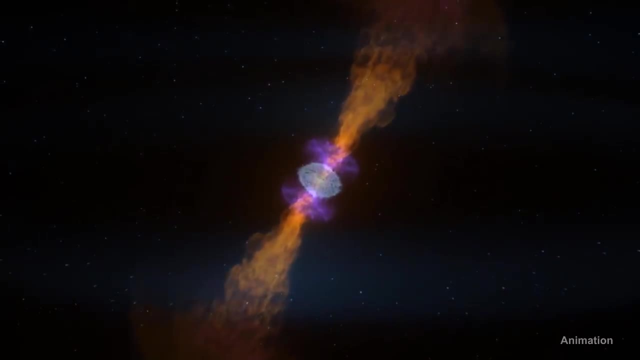 we noted, cosmic rays are produced in supernova, like the one that created the Crab Nebula. Gamma ray bursts are the most energetic and luminous electromagnetic events in the universe. They can release more energy in 10 seconds than our sun will emit in its entire 10 billion year. 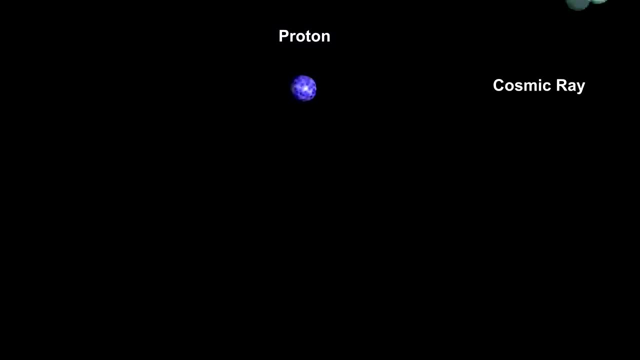 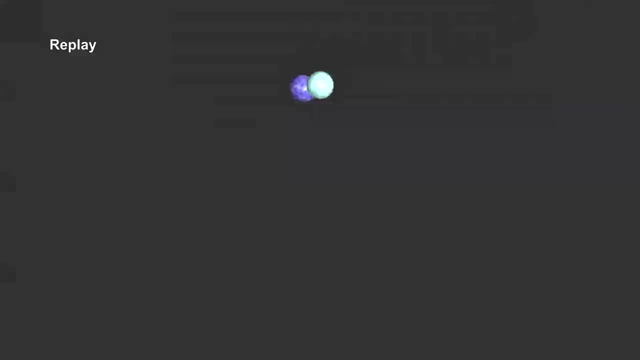 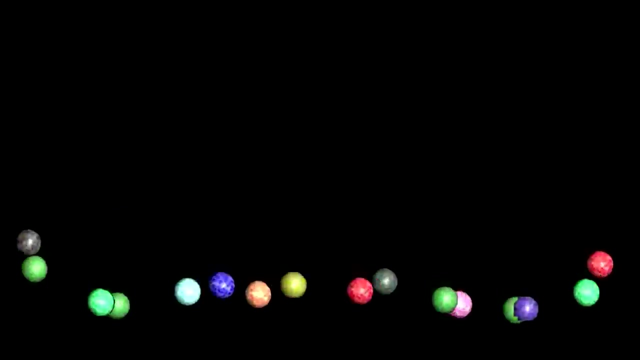 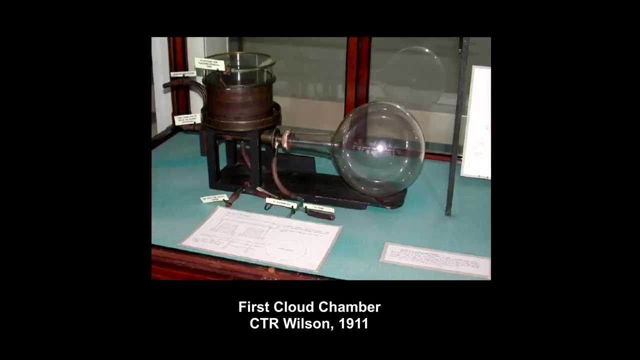 expected lifetime. It is the very high energy of the deep space cosmic rays that have the power to smash into electrons, protons and neutrons in the atmosphere, creating a wide variety of previously unknown particles. Charles Thomson Rees Wilson invented the cloud chamber in 1911 to detect these particles. 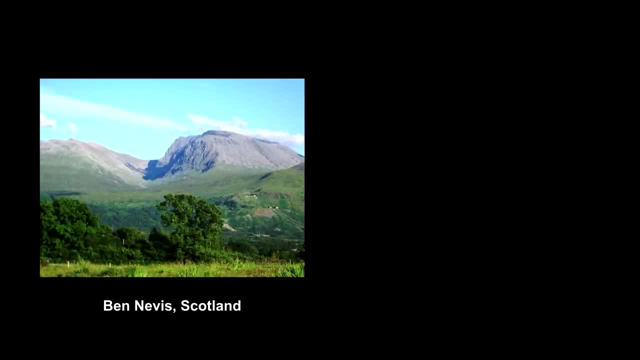 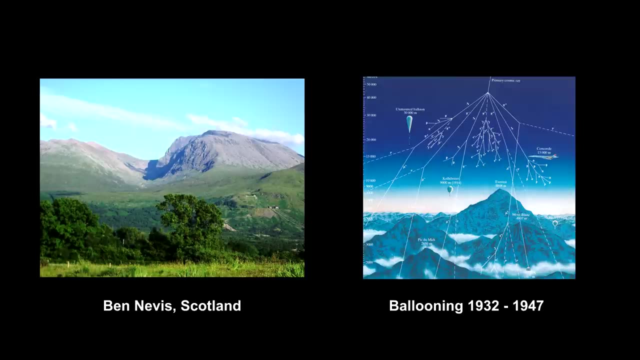 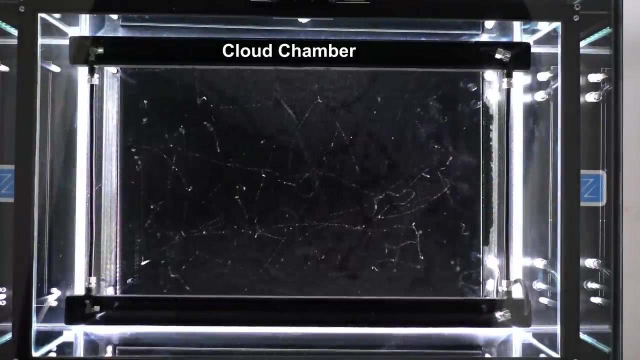 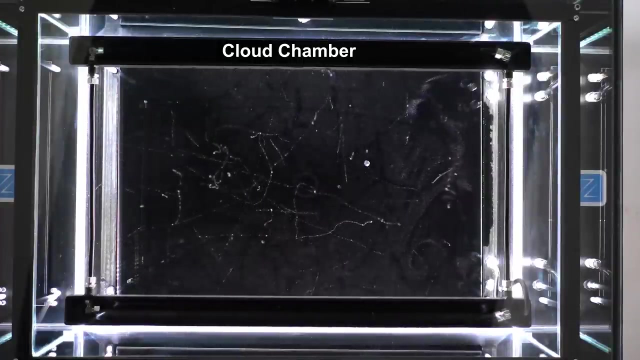 So physicists climbed mountains like this one that Wilson used and went up in balloons with their cloud chambers hunting for new particles. Here's what it looks like when charged particles pass through the atmosphere. The chamber contains a vapor of alcohol placed inside a magnetic field. When charged particles 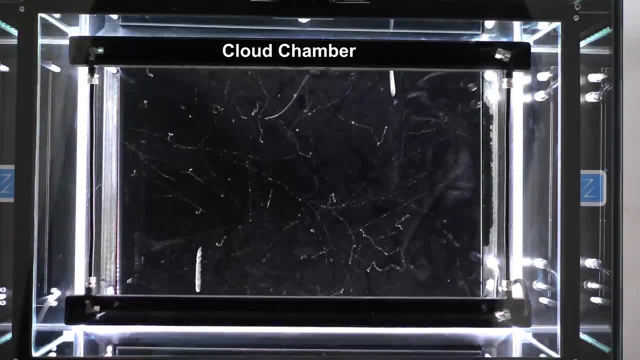 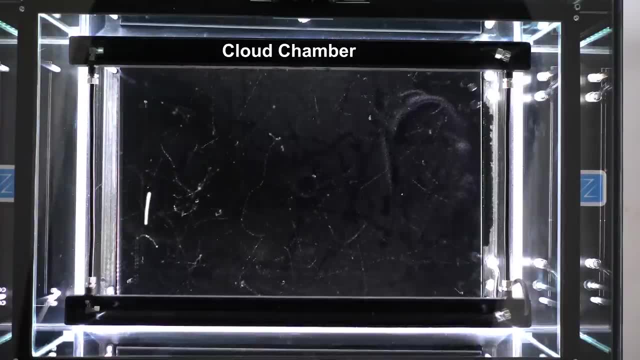 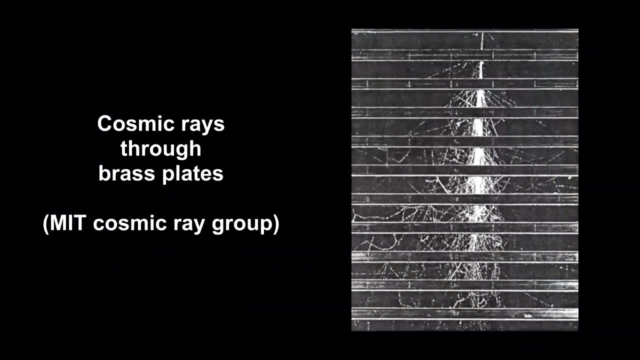 move through the chamber, they cause little droplets to form. These are the cloud tracks that we see. It works on the same principle as tracks forming behind high-flying jet aircraft. Here's what cosmic rays look like in a cloud chamber. These rays are penetrating multiple 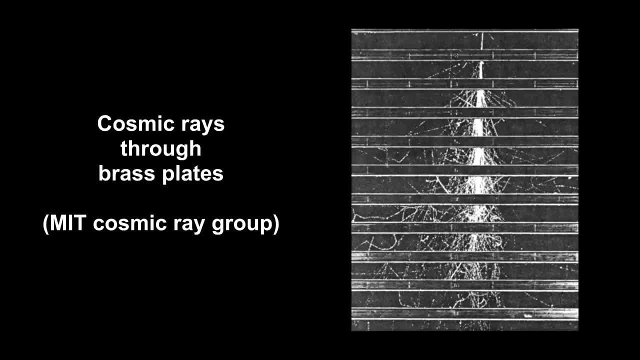 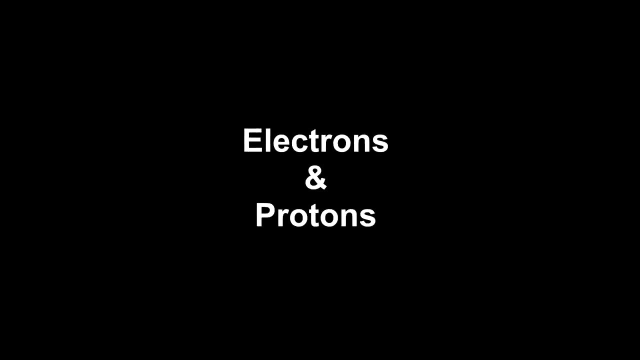 brass plates each 13 millimeters thick. To understand these tracks, we'll start with the two charged particles we already know: the electron and the proton. Here is a photograph of a particle track that is connected to the atmosphere. This is a. 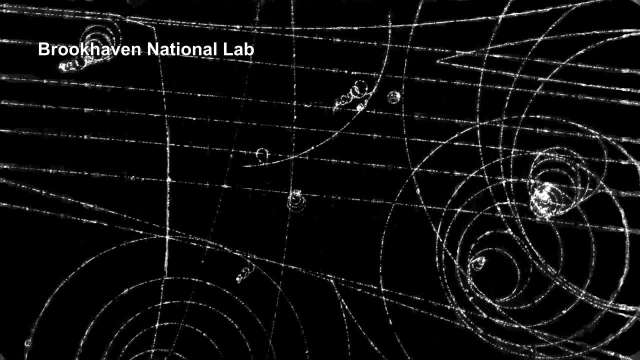 photograph of a particle track that is connected to the atmosphere. Here is a photograph of a particle track that is connected to the atmosphere. Here is a photograph of a particle track in a hydrogen bubble chamber from the Brookhaven National Lab, Given the direction of the. 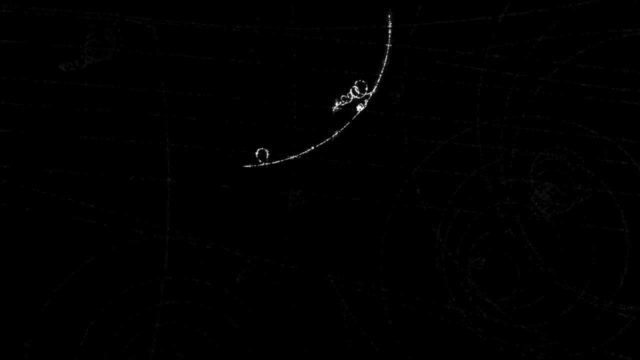 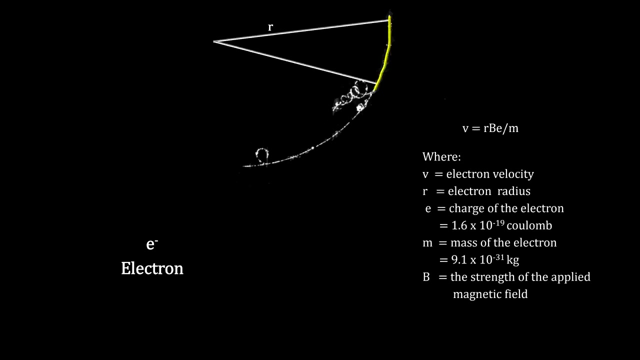 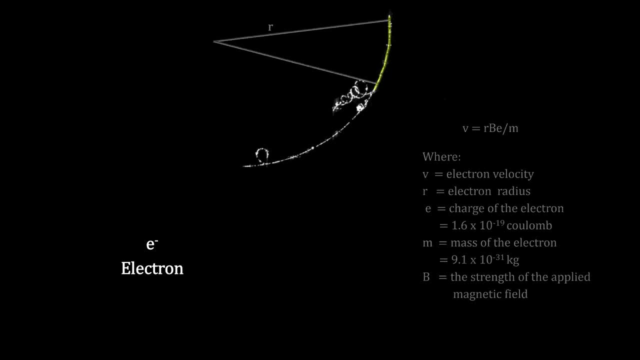 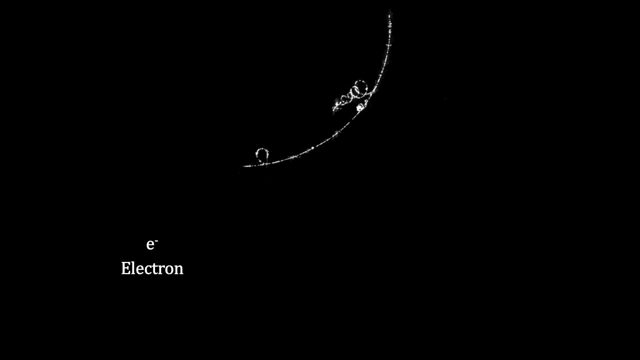 the electrons to slow down and their curvature to increase. At these three points we see that stationary electrons in our path have been bumped into motion. These are called knock-on electrons Because they are moving in a straight line. As they are moving very slowly, they spiral rapidly to a stop. 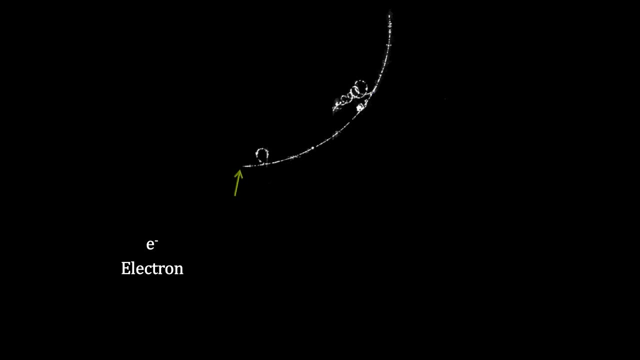 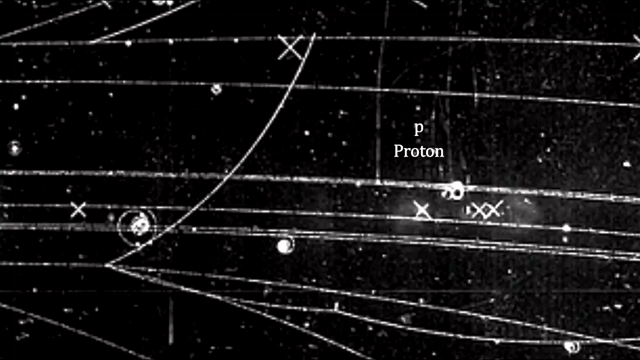 We see a lot of these in bubble chambers. The track ends when the electron is captured by a proton to form an electrically neutral hydrogen atom. In this bubble chamber photograph from CERN, we see a particle's track rotating counterclockwise. 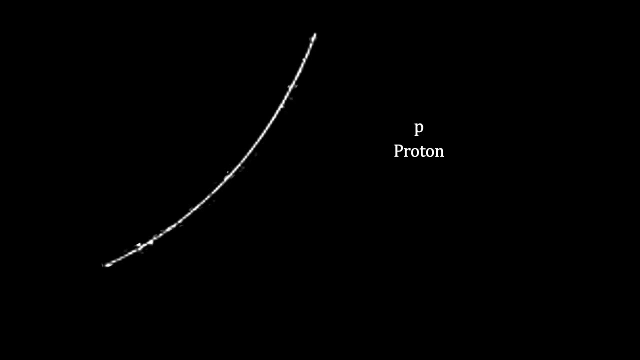 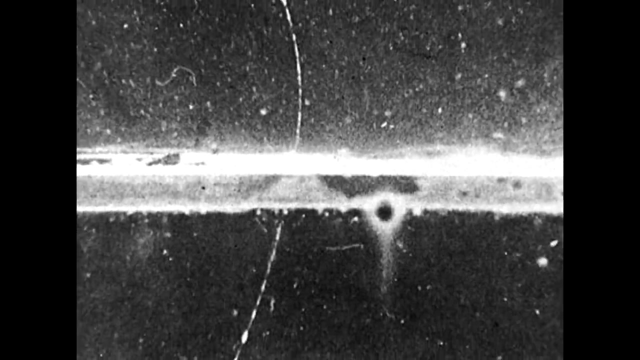 This indicates that it is positively charged. The particle's line is also thicker than the others. This indicates that it is a large, slow-moving particle. This is a characteristic of proton tracks. Now let's take a look at some of the new particles that sent the world of physics into. 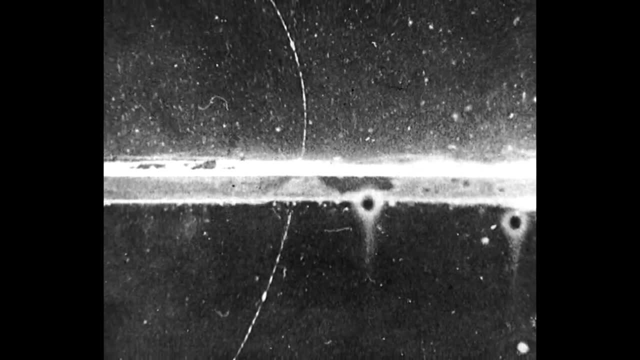 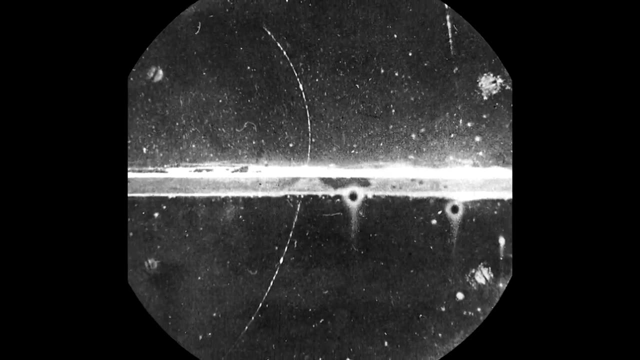 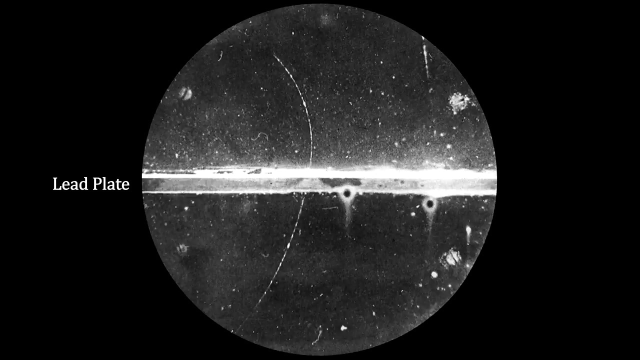 never-before-seen territory. In 1932, a new particle was discovered. In 1932, Carl David Anderson began investigations into cosmic rays and encountered unexpected particle tracks in his cloud chamber photographs. The 6 mm thick lead plate in the chamber is designed to slow particles down. 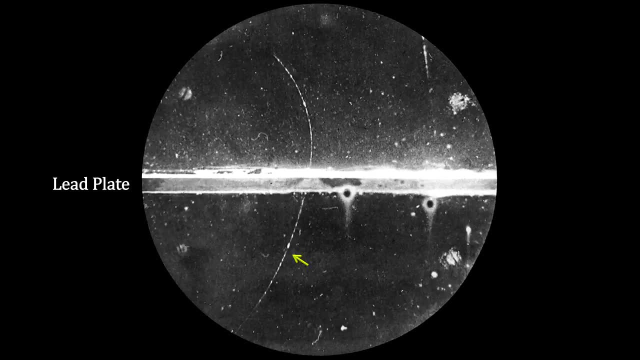 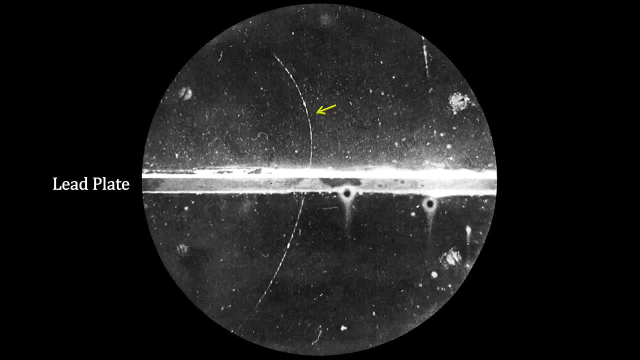 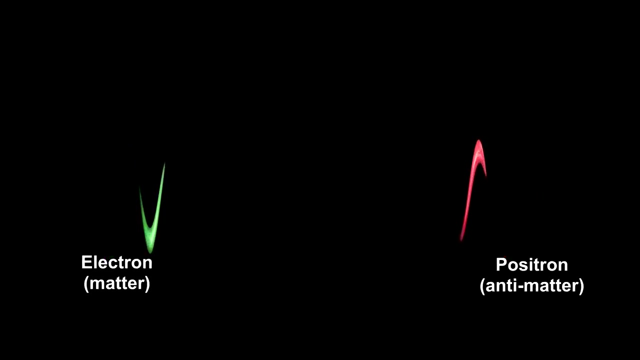 The particle is now moving at a slow speed. This curvature indicates that its mass is the same as an electron. This was the discovery of the positron. In 1928, four years before Anderson discovered the positron, Paul Dirac predicted the existence. 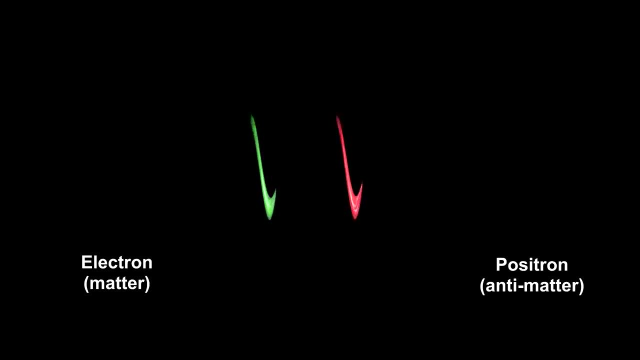 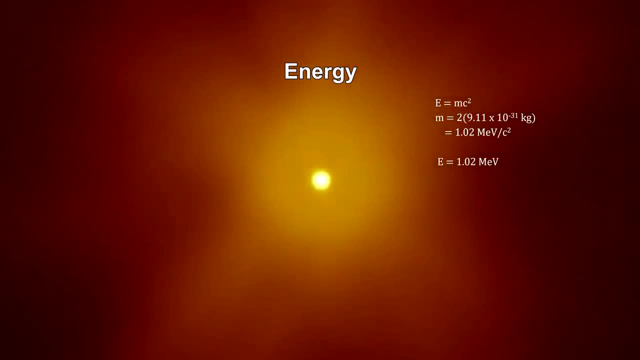 of antimatter and proposed that all particles had antiparticles and that they would annihilate each other if they came into contact with each other. bound each other and that they would annihilate each other if they came into contact. The positron is the antiparticle of the electron. 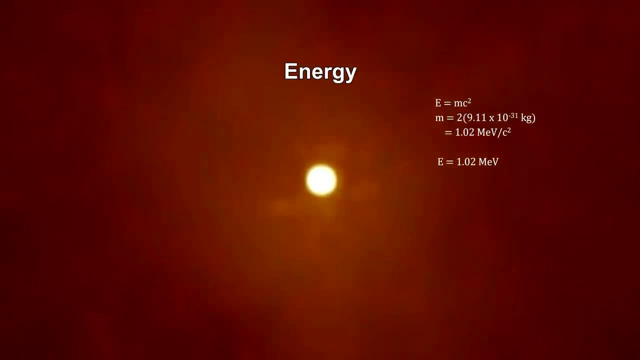 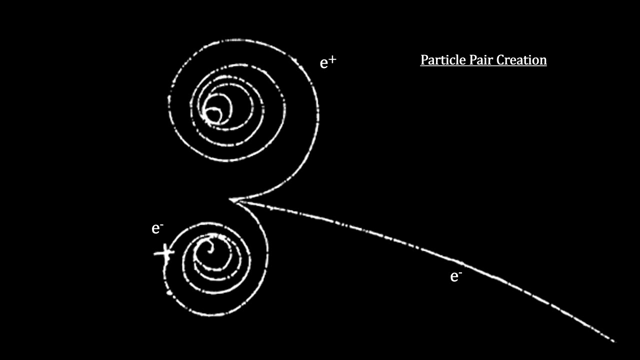 This is an example of converting matter to energy. Here's an event in a cloud chamber that shows the creation of a pair of particles, one electron and one positron, 사용 тонica. This event was the conversion of a high-energy gamma ray that can be switched between the appe informwiękäu. This event was the conversion of a high-energy gamma ray that can be switched between the 오른 birder neighbor plus daton Is the born 마음. so it is fantastic. This is called a南ij- extended mímt stiffness. 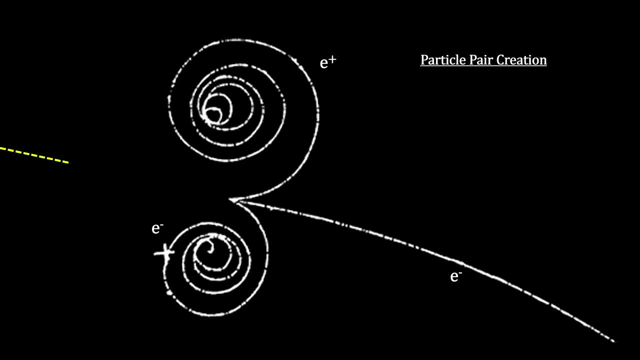 kicked an electron out of an atom and was itself converted into two particles. The gamma-ray photon does not show up in the cloud chamber because it has no charge. This is an example of converting energy to matter. The energy of the gamma-ray photon had to be as great as the energy embodied in the 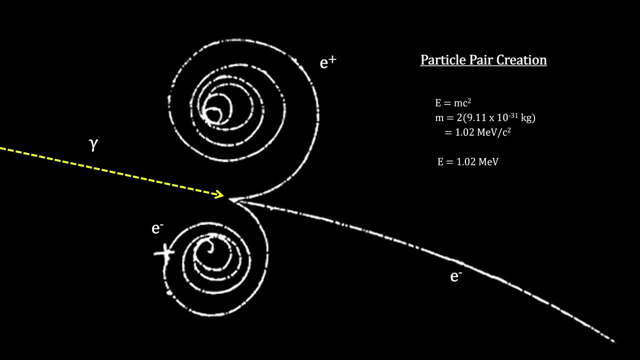 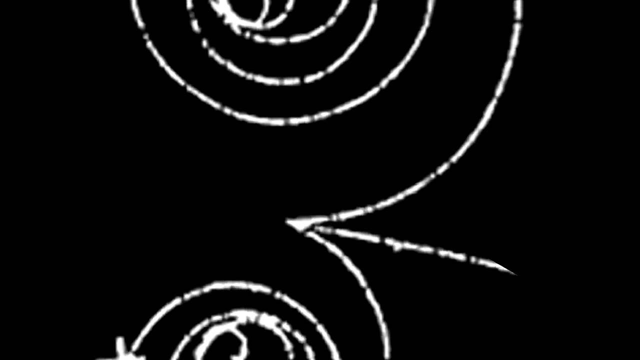 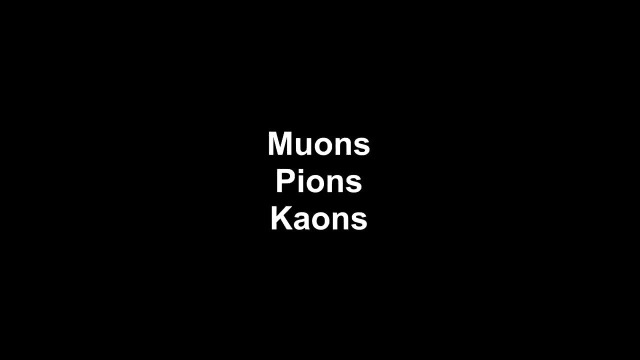 two particles For electrons and positrons, that comes to around a million electron volts. Any theory that attempts to explain this behavior will need to identify a way for energy, at any point in space, to create matter. In 1932, Paul Coons discovered the muon. 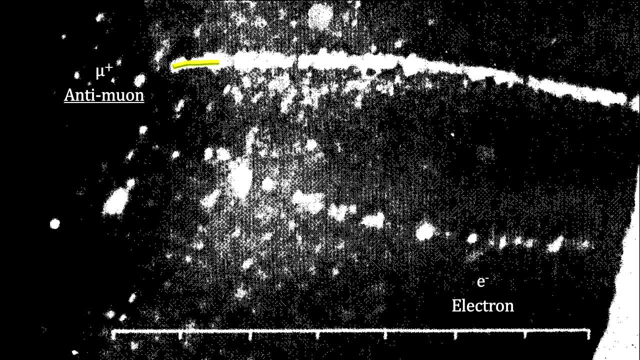 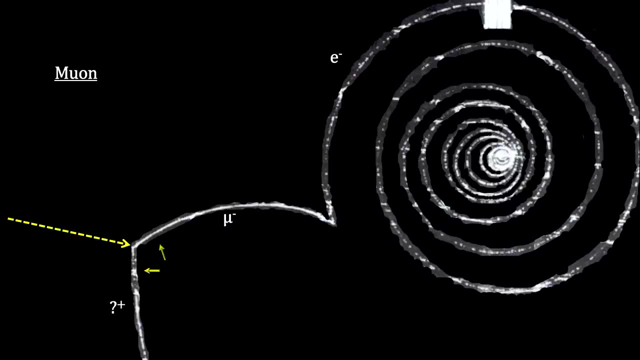 In the thickness of the bubble track. he calculated that it was a positively charged particle that was lighter than a proton but heavier than an electron. Later on it was found that this was the anti-muon. Here's another look at a muon created by an event that created two visible particles. 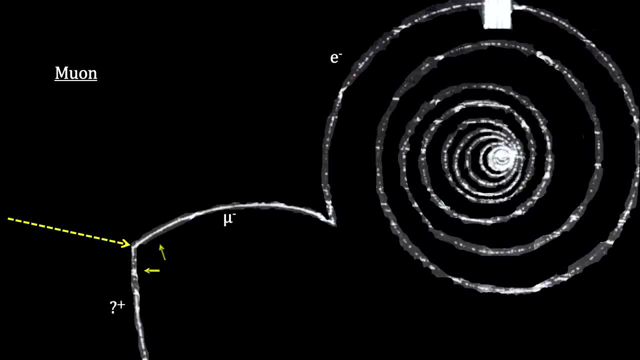 a muon and an unknown particle. The muon displayed a new particle property that had not been seen before: It was unstable, Unlike protons and electrons. the muon would only exist for a short period of time before it decayed into other particles. 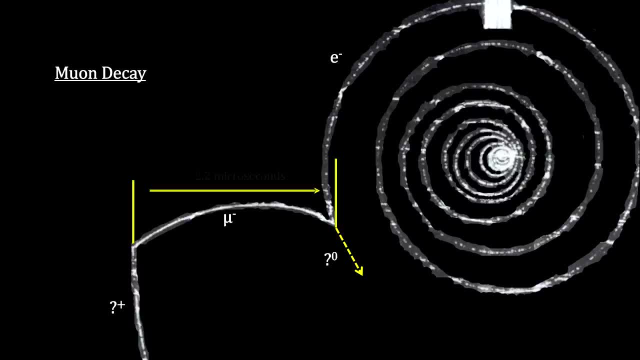 One was an electron and the other was unknown. On average, it lasted only 2.2 microseconds, That's 2.2 millionths of a second. Muons are light elementary particles like the electron and the positron. 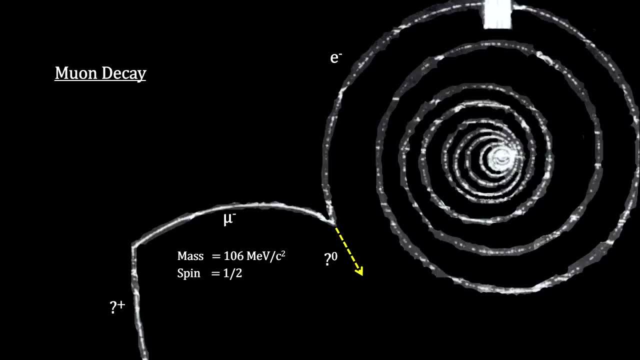 These particles are called leptons, meaning light rather than heavy like a proton. The particle that was created at the start, along with the muon, turned out to be the long-sought-after particle called the pion. In 1947,, using cosmic rays at high altitudes, the muon became a muon. 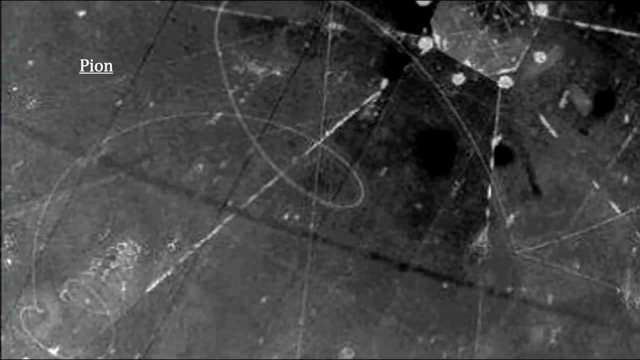 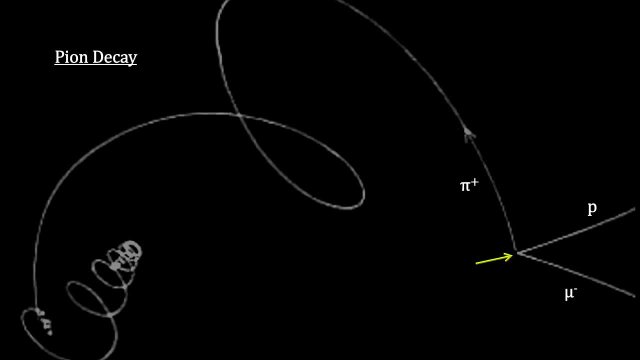 The muon became a muon. When the muon decays at high altitudes, this particle was found Here. we see an event that kicks a proton into motion and creates a muon and a pion. Then we see the pion decay into an anti-muon that itself decays into a positron. 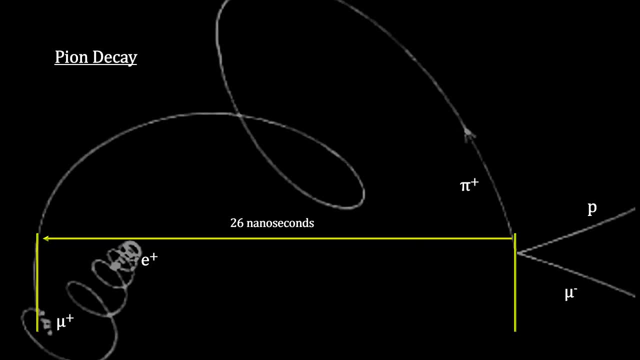 It lasted only 26 nanoseconds. Now, that is a very short life. The muon lasted almost a thousand times longer than that. Pions are spin-zero particles with around 14 hundredths of a proton's mass. Although that's small, it's a good deal more massive than the muon. 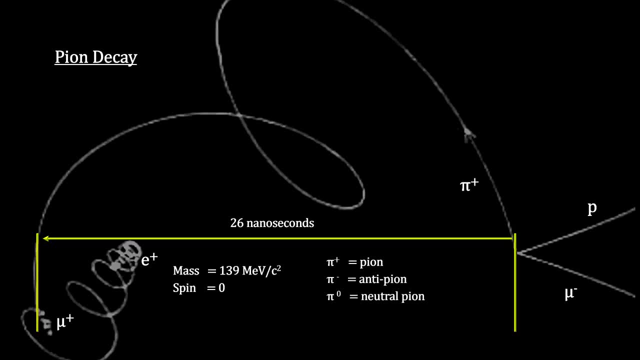 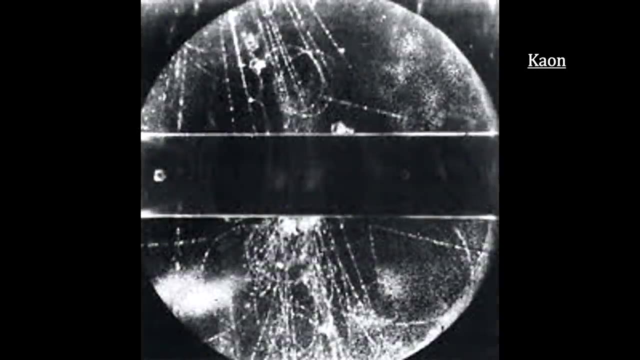 Pions came in three flavors: one with a positive charge, one with a negative charge called the antipion, and one with no charge at all. Also in 1947, another particle called the kaon was discovered by George Rochester and Clifford Butler. 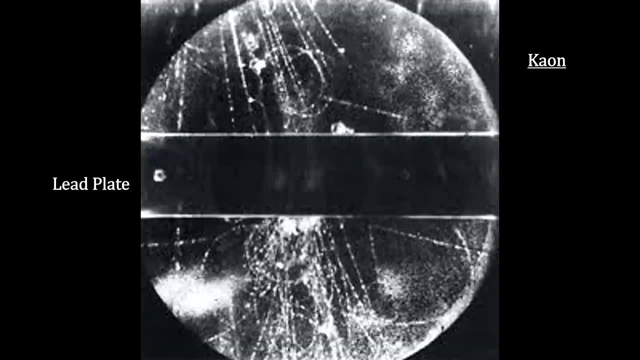 They also used cosmic rays. Here's a look at their bubble chamber picture. Just below the lead plate in the lower right hand quadrant you see an inverted V that extends to the lower right, Measuring the momentum and charges. they determined that they were a pion and an antipion. 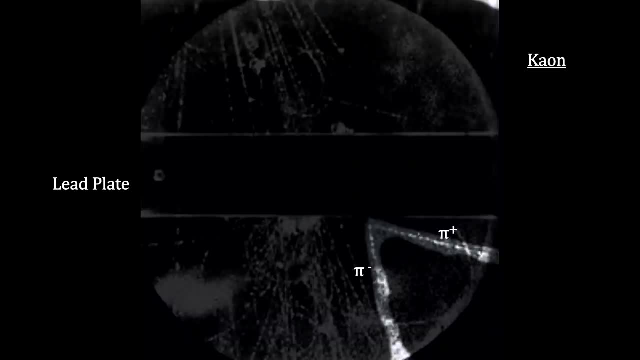 Rochester and Butler concluded that this event had to be a photographic record of a novel phenomenon: the decay of a previously unknown neutral heavy particle, later called the kaon. The discovery of kaons represented the first time we deduced the existence of a particle. 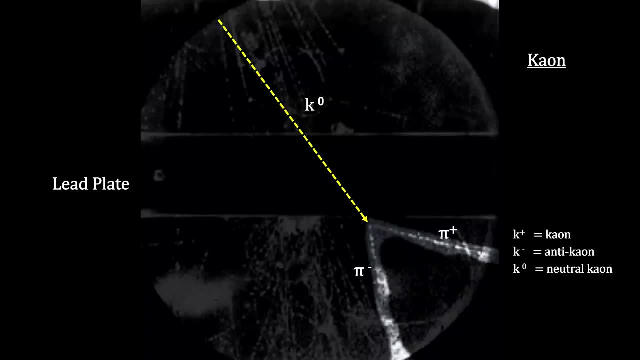 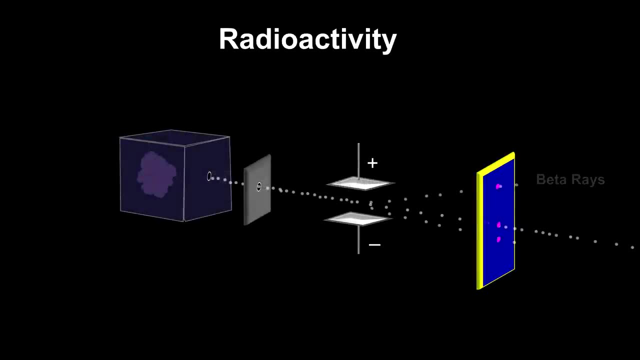 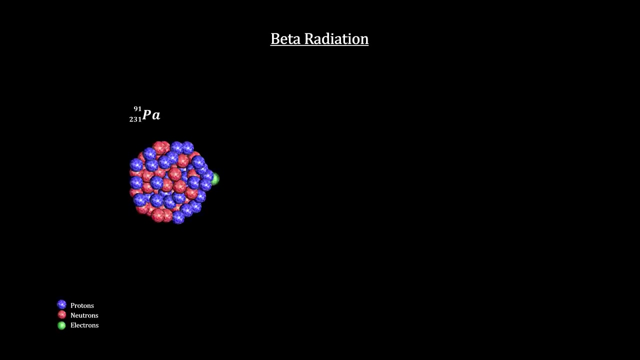 from its decay. One of my favorite particles is the neutrino. You'll recall from our segment on radiation that the beta rays were ejected electrons. What's happening here is that a neutron inside the nucleus of an atom is spontaneously decaying into a proton and ejecting an electron in the process. 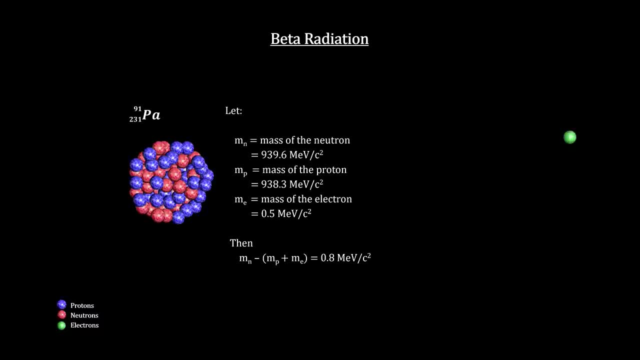 The mass of the proton plus the mass of the electron is less than the mass of the neutron, And because energy is conserved, some energy must be released to make up for the difference. From Einstein, we know that energy equals mass times the speed of light squared. 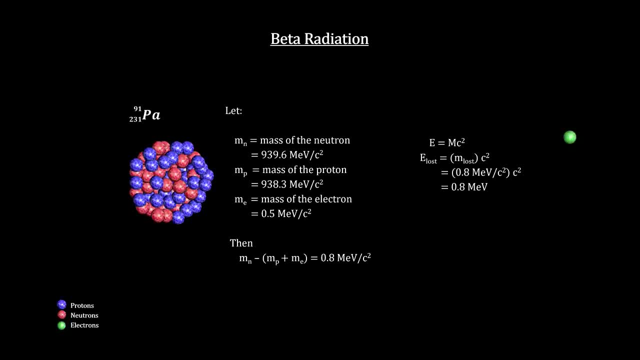 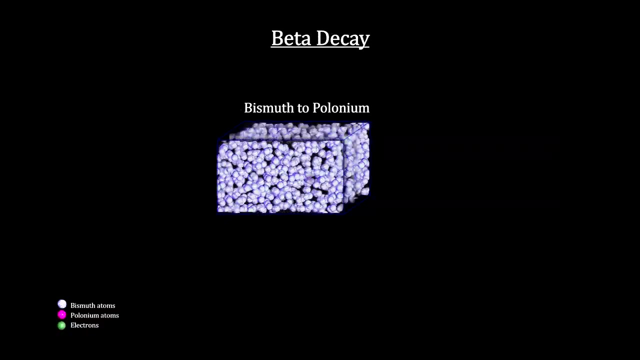 So if the lost mass is turned into energy, we can calculate the amount: Just under a million electron volts per atom. It was assumed that this energy was accounted for by the kinetic energy of the ejected electrons. In 1927, two physicists, CD Ellis and WA Worcester, set out to measure this energy. 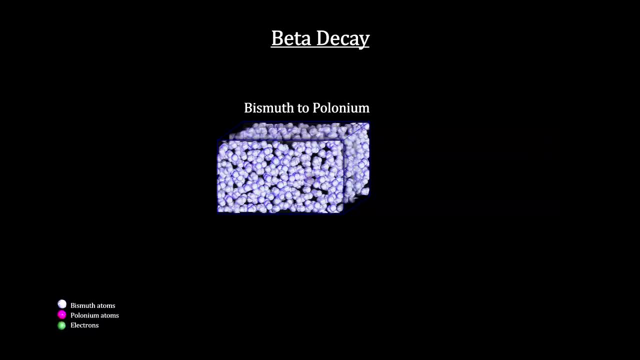 They used bismuth 210, a product of radium decay that itself decays into polonium. The rate at which unstable radioactive nuclei decay in a sample is called the activity of the sample. The greater the activity, the more nuclear decays per second. 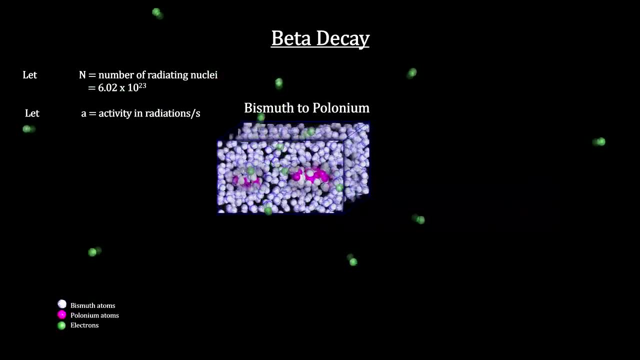 This is rather easily measured with devices like a Geiger counter. Given the number of radiating molecules in a sample and measuring the activity, we can calculate the probability for any one molecule to decay in a second. This is called the decay constant. 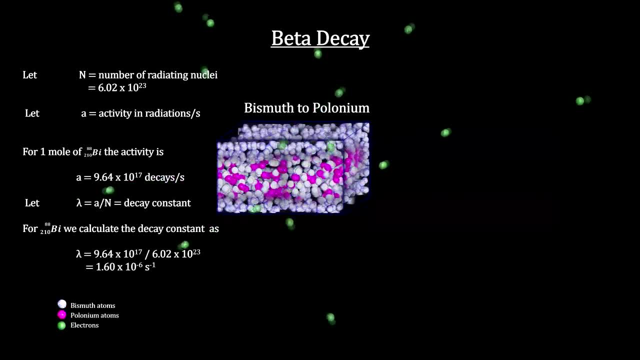 We find that the decay constant is always a small number, constant over time and different for different materials. Both the activity rate and the number of radioactive nuclei vary over time. As a sample decays, the number of radioactive nuclei decreases, With fewer radioactive nuclei. 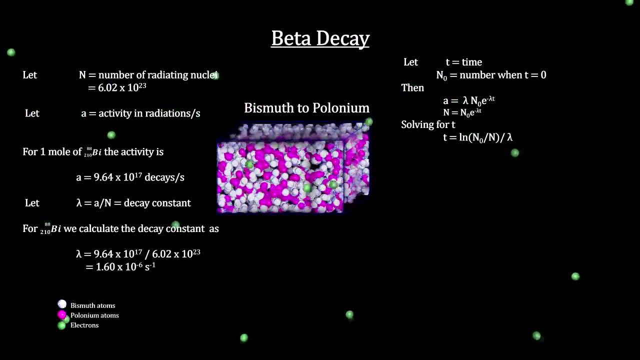 the activity rate also decreases. From this we get the exponential law of radioactive decay. It tells us how the number of radioactive decay in a sample decreases with time. The half-life is the time it takes for the material and activity to be reduced by half. 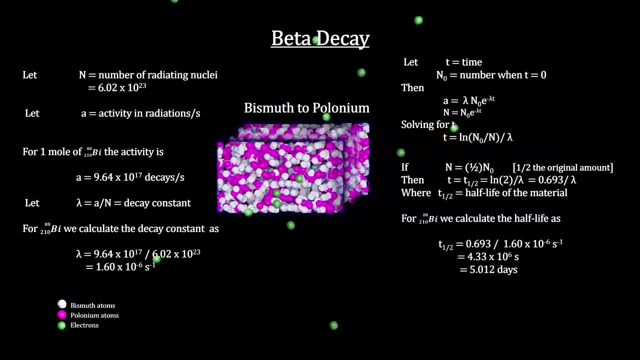 Bismuth 210 has a half-life of five days, meaning it takes five days for half of any amount to transform into polonium. We cover half-life in more detail in the How Old is the Earth-Moon System segment in the How Old Is It video book. 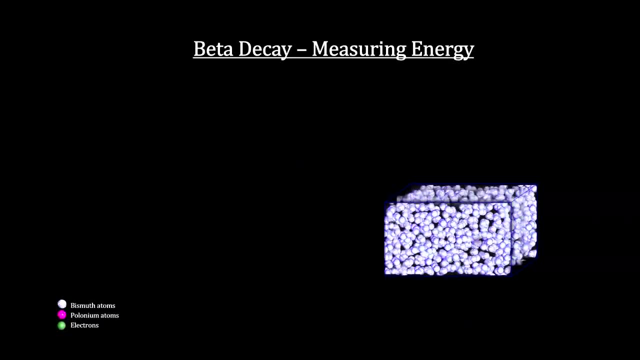 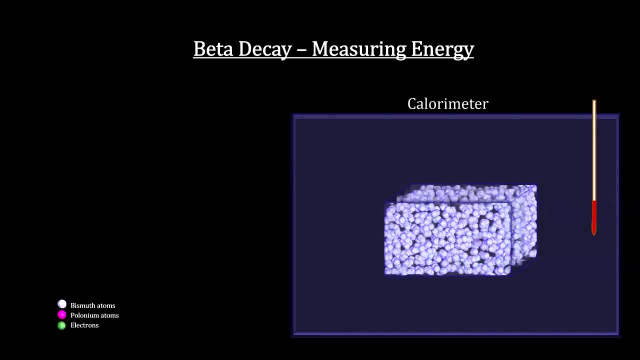 The experiment was simple: Place the bismuth into a calorimeter. The calorimeter keeps the energy of the beta radiation inside the container Over the five days. each and every ejected electron's kinetic energy is converted to heat as they collide with the water molecules. 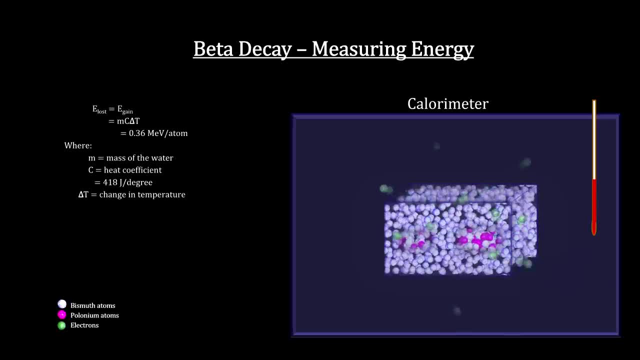 and come to rest in the calorimeter. Measuring the change in temperature allows us to calculate the amount of energy absorbed. The results showed that each bismuth atom naturally emits 0.36 million times, That's more than twice as much as was measured. 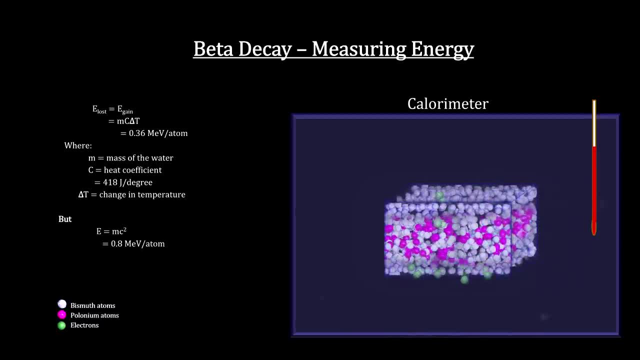 But here we had a significant discrepancy. Conservation of energy and Einstein's equations called for 0.8 million electron volts, That's more than twice as much as was measured. This was a real problem. Niles Bohr thought that the conservation of energy didn't hold in this case. 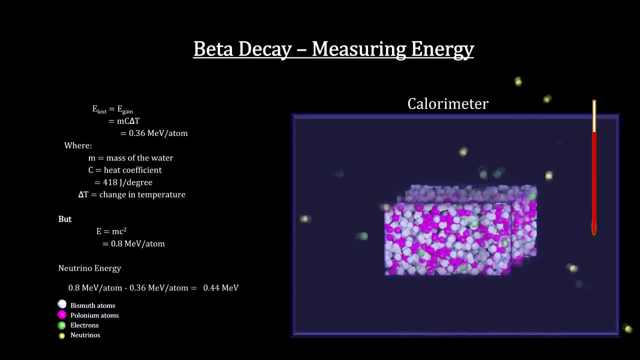 while Wolfgang Pauli thought that it did and proposed that there must be another particle that doesn't interact much with its surroundings and carried away the missing energy. In 1931, Enrico Fermi named Pauli's particle the neutrino, or a small neutral particle. 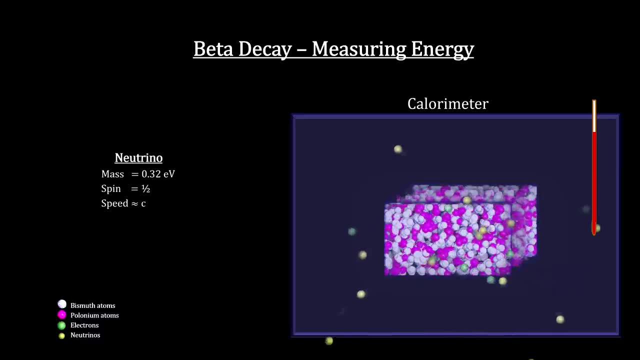 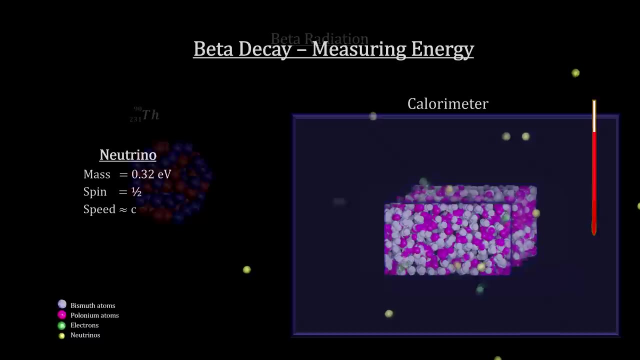 The neutrino's predicted mass was around a third of an electron volt. This is over a million times smaller than the electron. Its predicted spin was one half and its predicted speed was almost the speed of light. This would have beta radiation look like this: 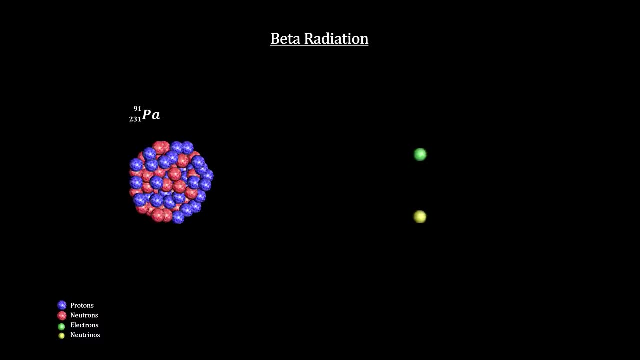 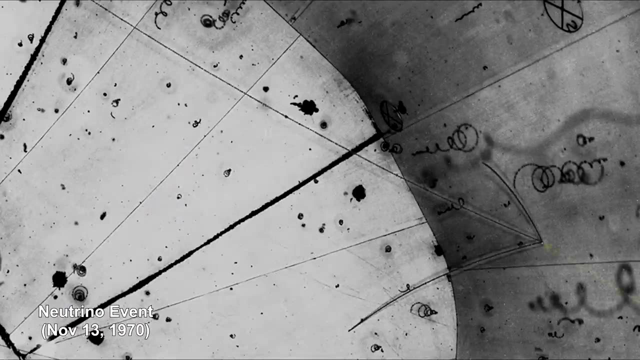 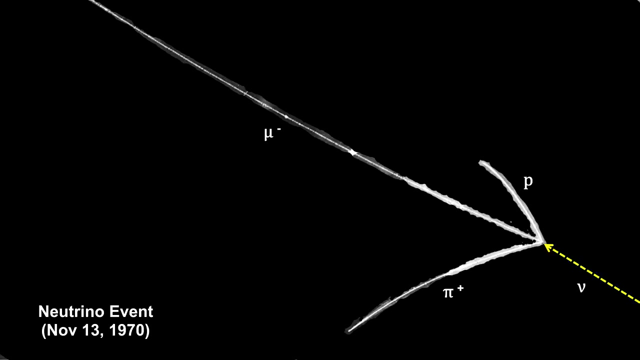 with both an electron and a neutrino being ejected. This particle was finally observed in a hydrogen bubble chamber captured in 1970.. The invisible neutrino enters from the lower right and strikes a proton where the three-particle tracks originate. The proton is kicked into motion. 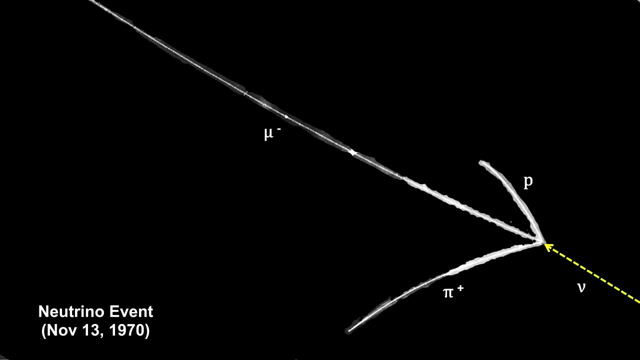 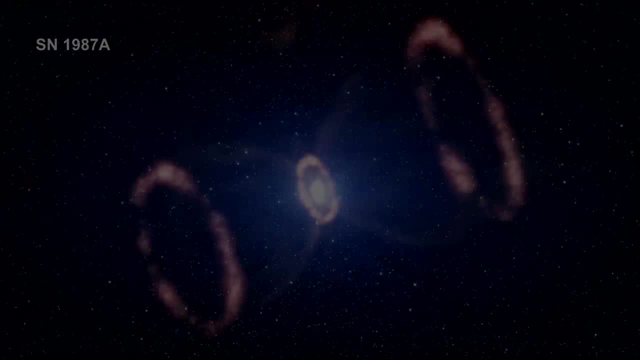 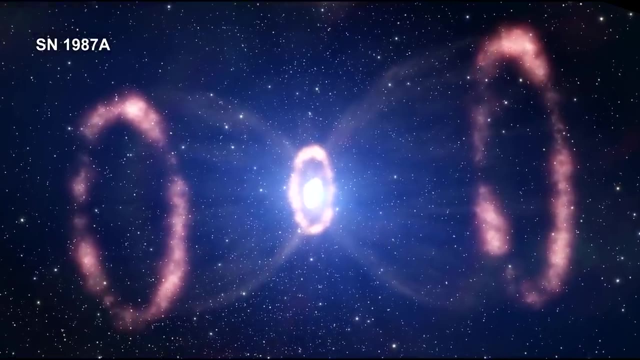 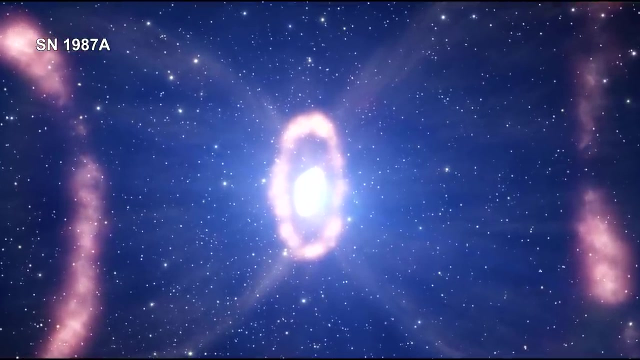 and the neutrino is converted into a muon and a pion by the power of the collision with the proton. The neutrino is a critical component in many nuclear reactions that occur in stars. The detection of solar neutrinos and of neutrinos from supernova 1987A. 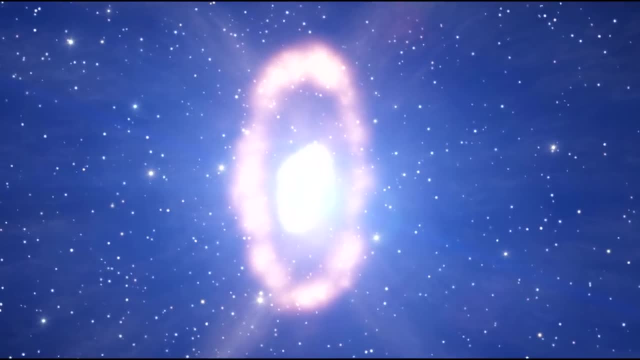 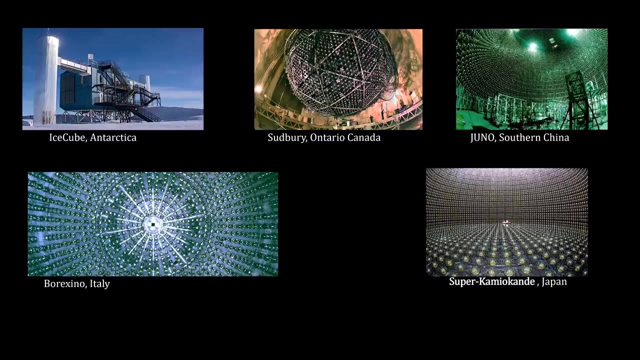 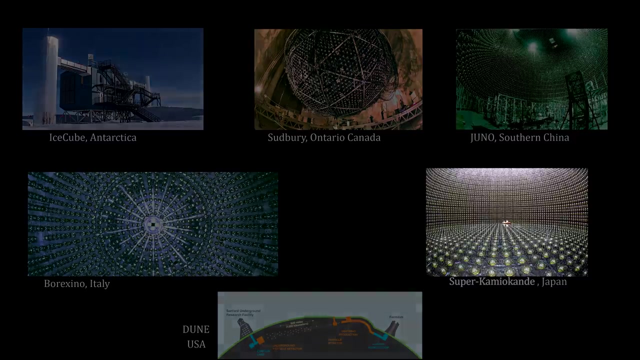 marked the beginning of neutrino astronomy. Today, there are a number of neutrino observatories in operation around the world and one under construction, to better understand these fundamental but elusive particles. We'll take a closer look at one of them, the Super Kameikande. 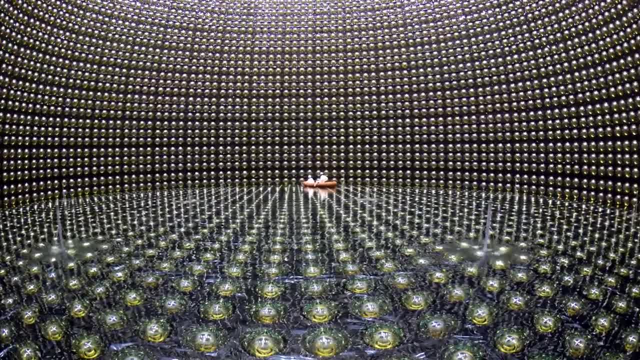 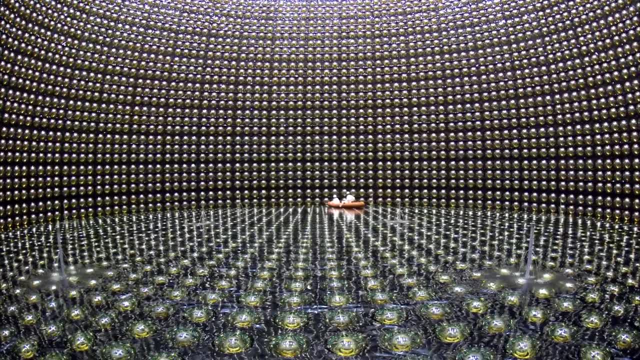 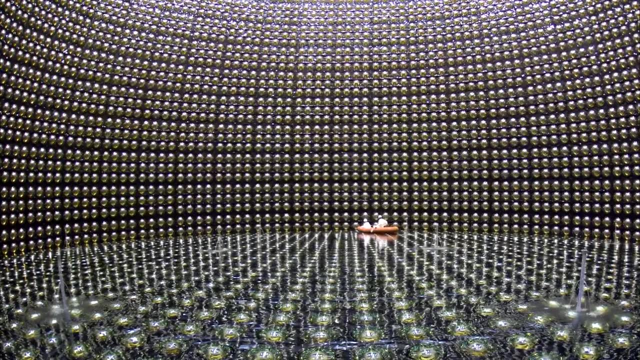 located 1,000 meters underground in a Japanese mine. It contains a lake holding 50,000 tons of ultra-pure water, surrounded by an inner detector with over 11,000 photomultiplier tubes and a flash when struck by a photon. 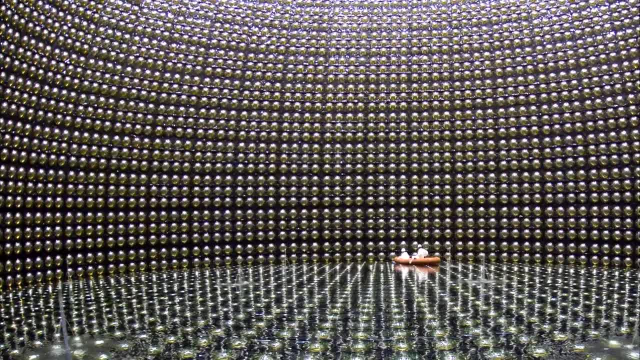 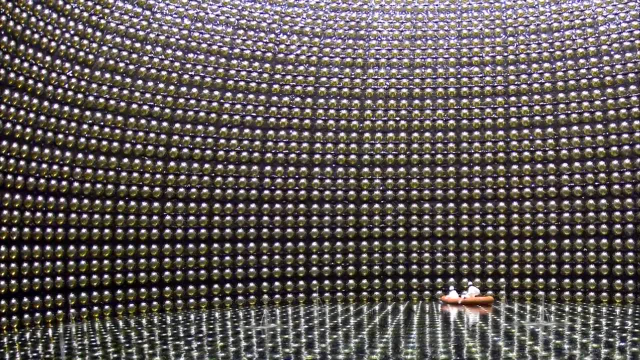 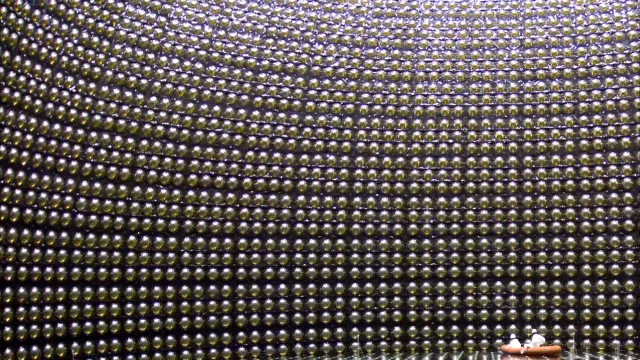 created by a neutrino interaction with the water. The speed of light in water is slower than the speed of light in a vacuum. A neutrino interaction with the electron or nuclei of water can produce a charged particle that moves faster than the speed of light in water. 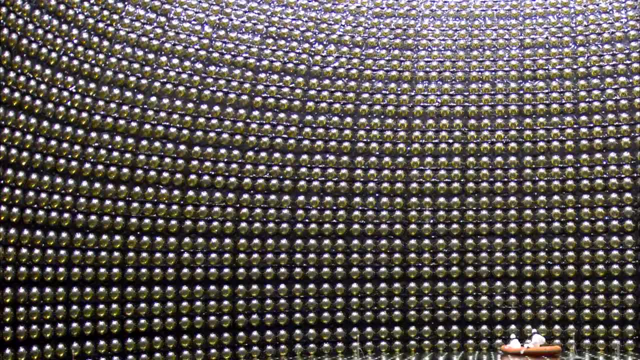 This creates a cone of light known as Chernikov radiation. This is the optical equivalent of a sonic boom. The Chernikov light is projected as a ring on the wall of the detector and recorded by the photomultipliers. This figure shows the Sun. 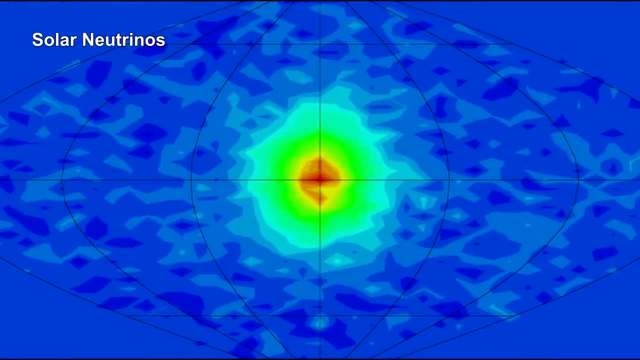 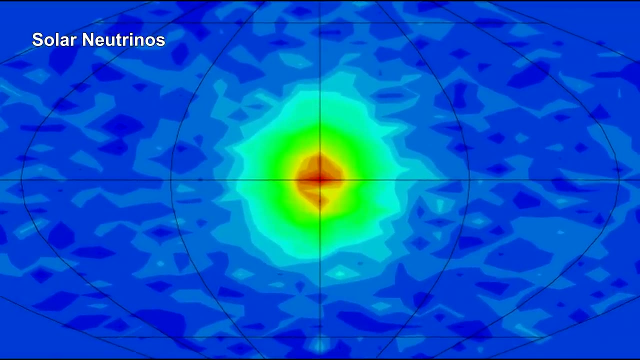 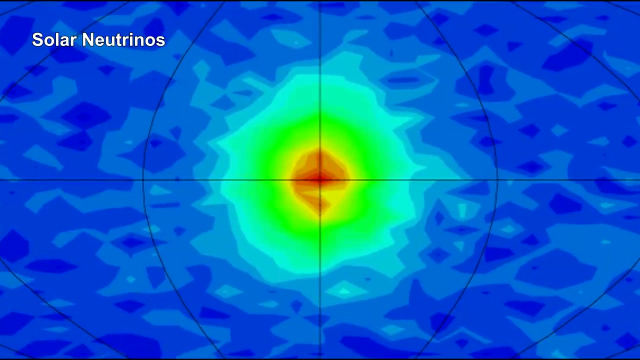 as observed by Super Kameikande, The Sun sends about 65 billion neutrinos per square centimeter our way every second. That's over 400 billion neutrinos per square inch per second. That's a lot of neutrinos, And almost all of them pass right through the Earth. 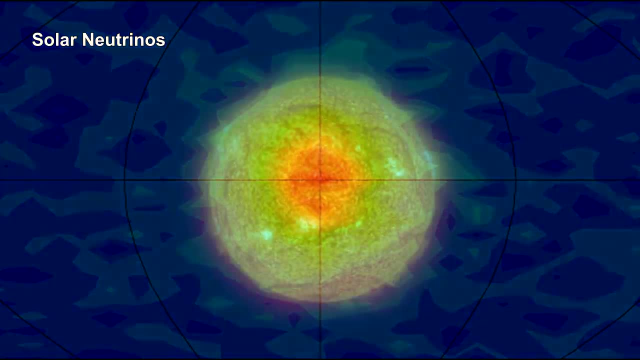 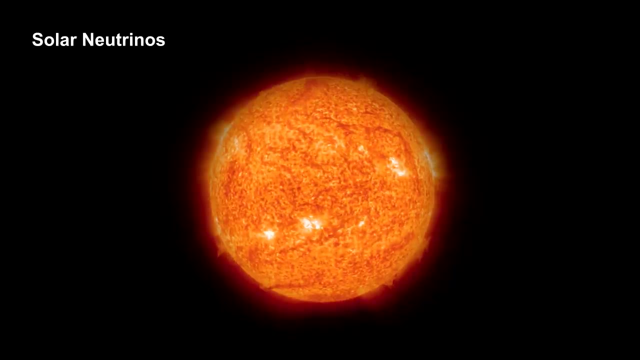 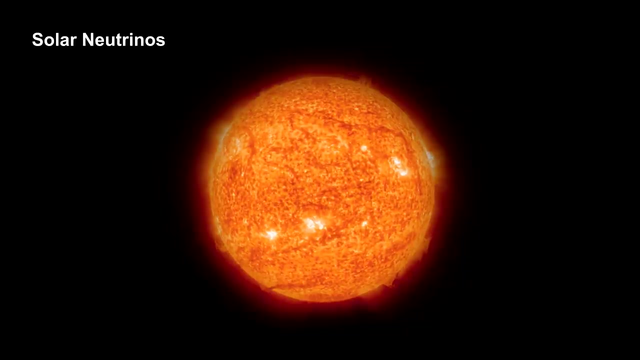 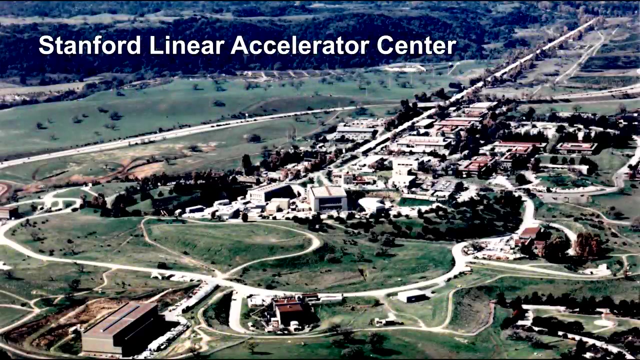 and out the other side. Trillions of neutrinos are passing through your body every second. I think that neutrinos will wind up playing a significant role in our understanding of dark matter. In 1969, a team of scientists at the Stanford Linear Accelerator Center. 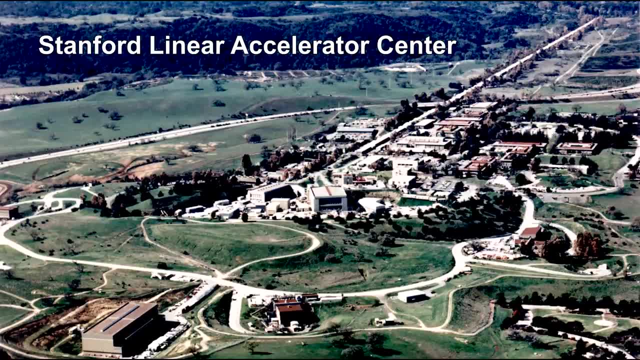 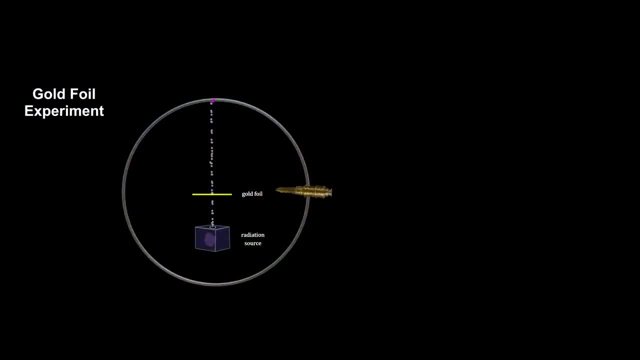 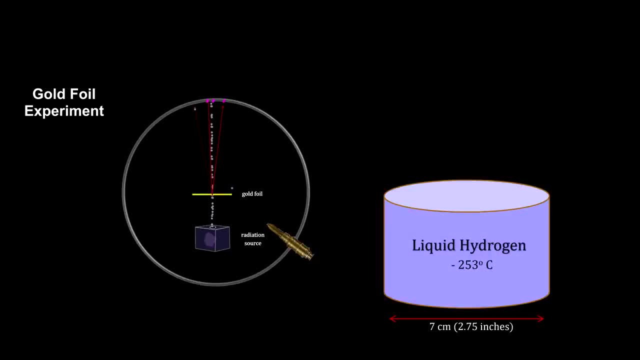 or SLAC for short, in conjunction with MIT, performed scattering experiments similar in principle to what Rutherford did to probe the atom 58 years earlier. Rutherford's target was a gold foil. In the SLAC experiment, the target was liquid hydrogen. 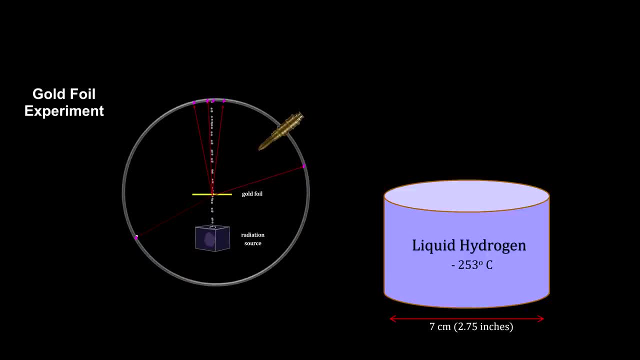 at a very cold temperature to keep the protons as close together as possible. As a source, Rutherford used a small piece of radium. The energy of the naturally occurring alpha particles was 7.7 million electron volts. Here we use electrons. 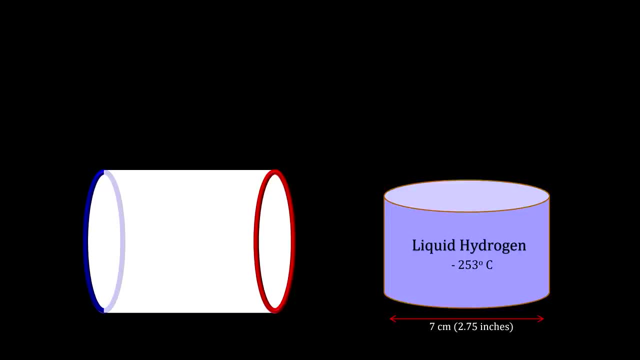 and accelerate them to nearly the speed of light. To do that we construct a glass tube. Then we connect a negative charge to the entrance and a positive charge to the exit. When the battery is turned off, electrons flow in any direction, But with the battery turned on, 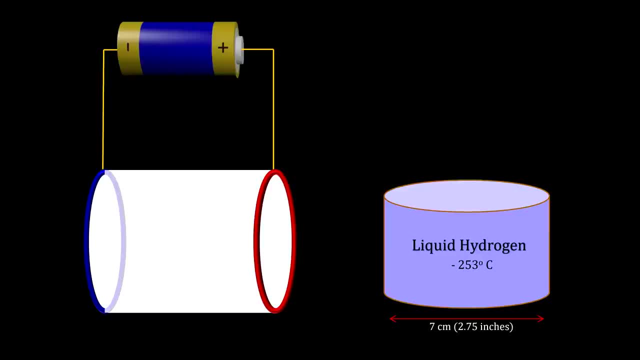 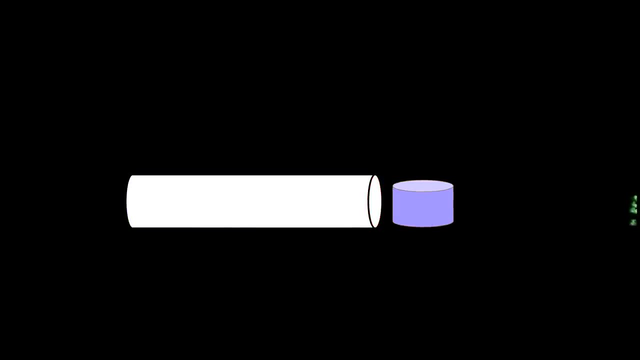 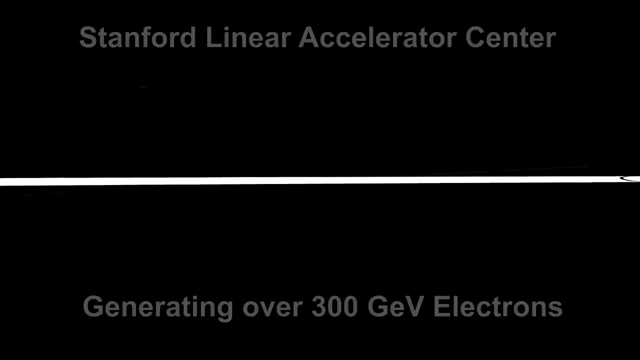 the electrons accelerate down the tube along the electric field To get a really high velocity. we connect more and more of these tubes together. At SLAC, the length of the tube is 3 kilometers, That's 1.86 miles. This creates electrons with 40,000 times the energy. 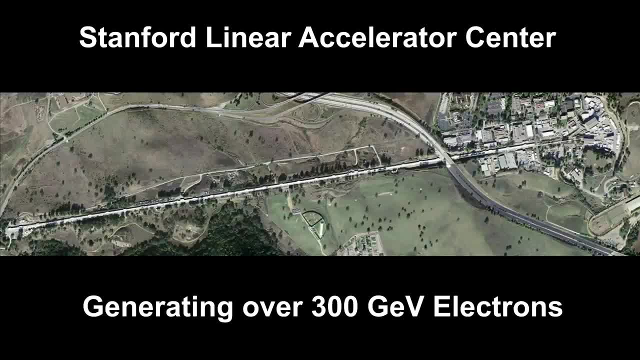 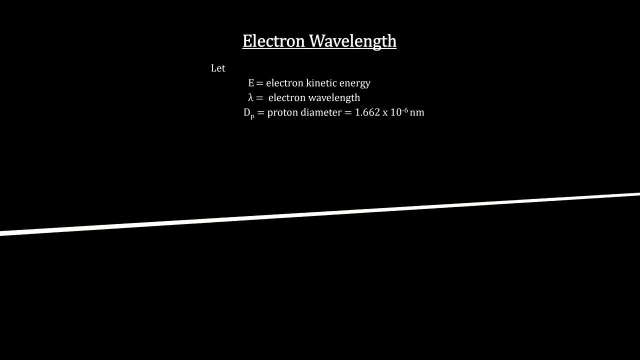 than the alpha particles used by Rutherford. This high energy is essential. You cannot probe inside a proton with a large wavelength electron. Remember that the wavelength of an electron in its ground state around a hydrogen nucleus is 200,000 times larger than the diameter of a proton. 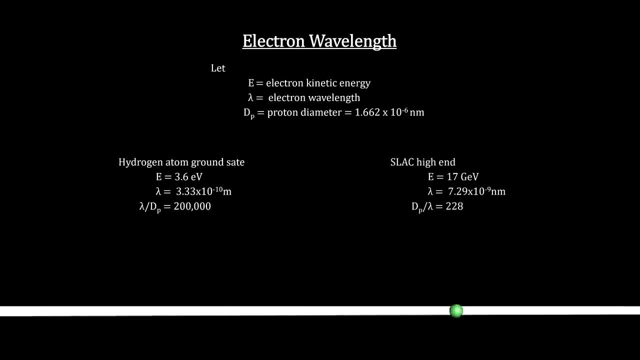 But if an electron's velocity is large enough, making its de Broglie wavelength small enough, it can. SLAC accelerates electrons to greater than 99.999% of the speed of light, creating a wavelength of the electron that ranges from: 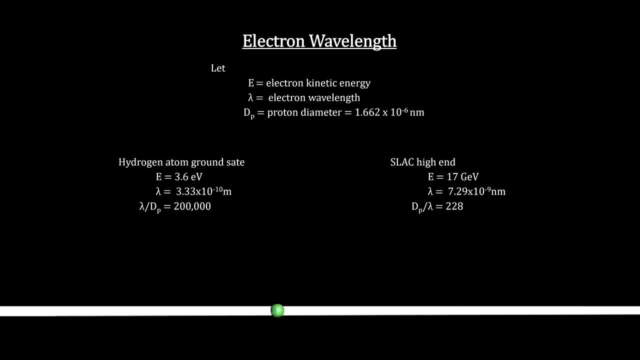 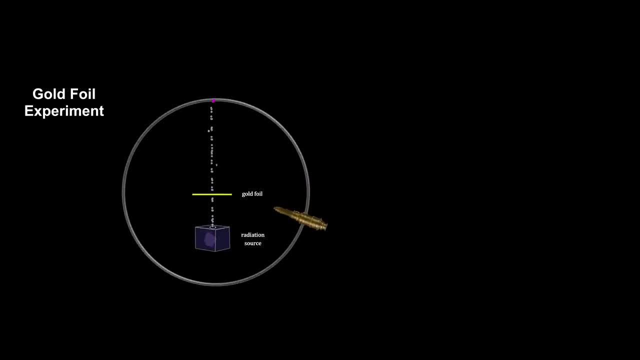 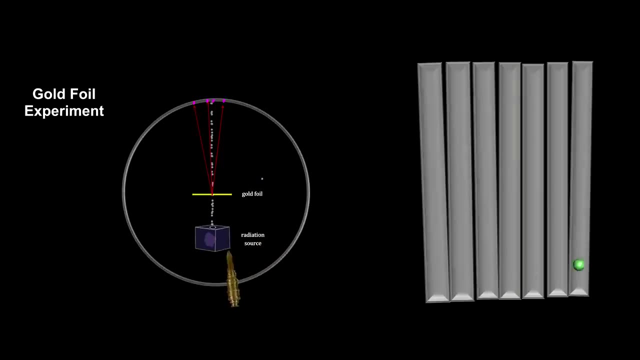 2 to 200 times smaller than the proton. The scintillator screen used by Rutherford covered the inside of the apparatus. He had to manually note the flash locations as he viewed them through the swiveling microscope. At SLAC we partitioned the scintillator screen into small strips. 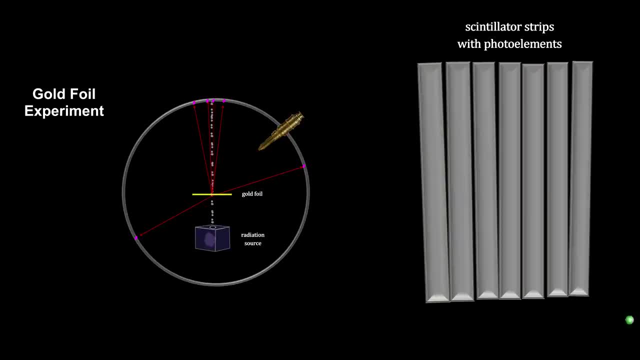 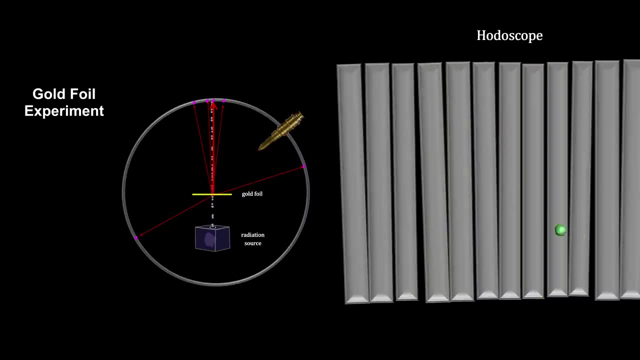 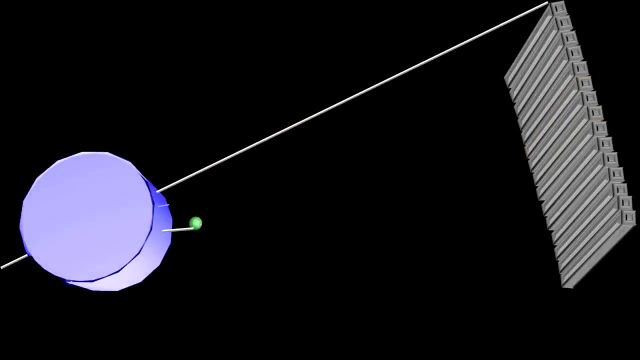 Each strip has an attached photo element that converts the flash into an electrical signal. This enables the sending of electronic location coordinates to a computer. This is called a hodoscope. With this we can precisely measure the scattering angles as the high energy electrons penetrate the hydrogen atom. 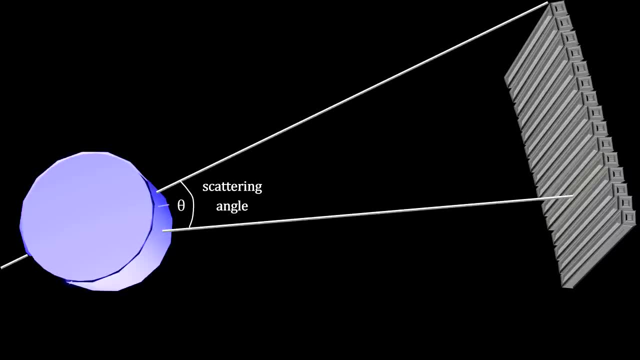 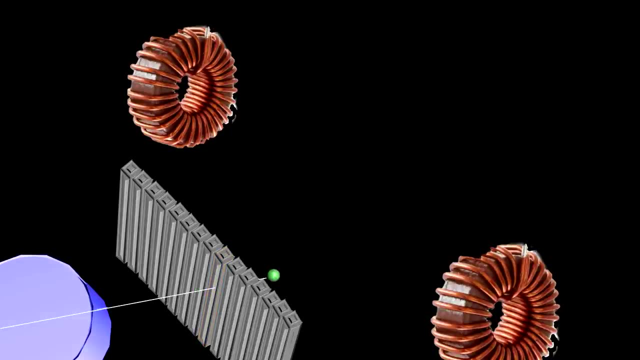 and approach the proton at the center. SLAC also introduces a strong magnetic field that will cause the scattered electrons to curve as they pass through. As you'll recall, from mass spectrometer and bubble chamber analysis techniques, the measured curvature will give us the momentum and velocity of the electrons. 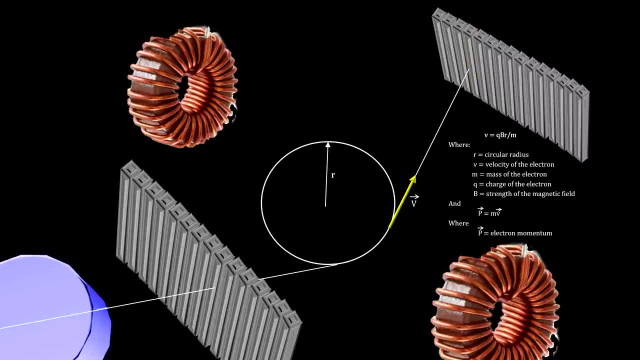 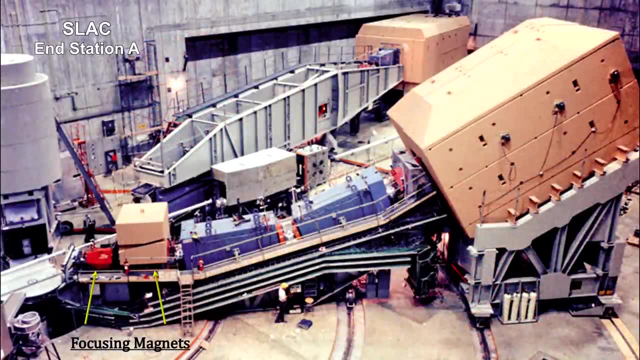 To measure this, a second hodoscope is installed at an angle. At the end of the process. the electrons enter a calorimeter that will measure its energy, much like we just did to discover the neutrino. Putting all these pieces together gives us the complete linear accelerator detector. 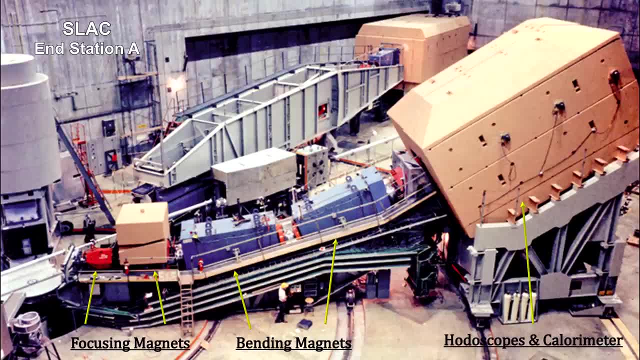 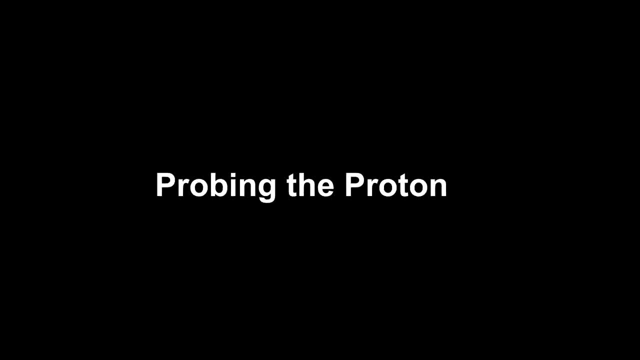 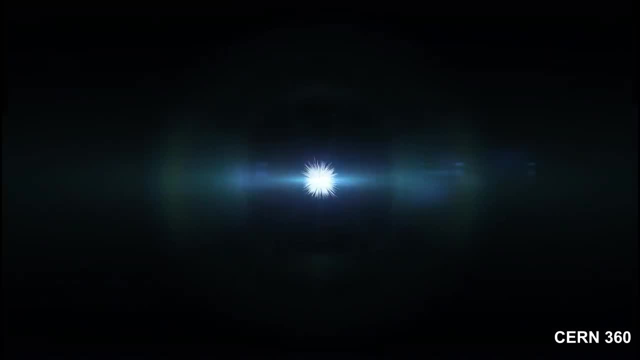 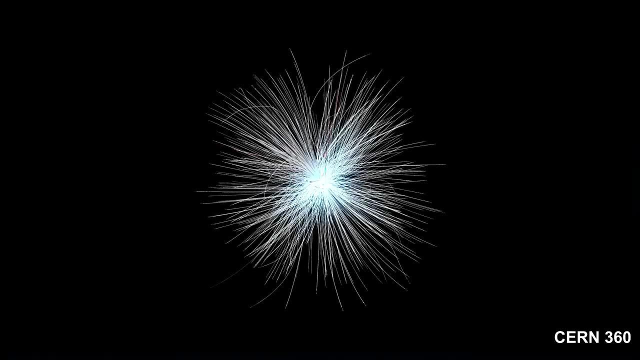 It weighs 750 tons. The Stanford linear accelerator was built to probe the proton with electrons, like Rutherford probed the atom with alpha particles. They both used scattering techniques. These techniques are key to understanding how the Higgs particle was found at CERN in 2012.. 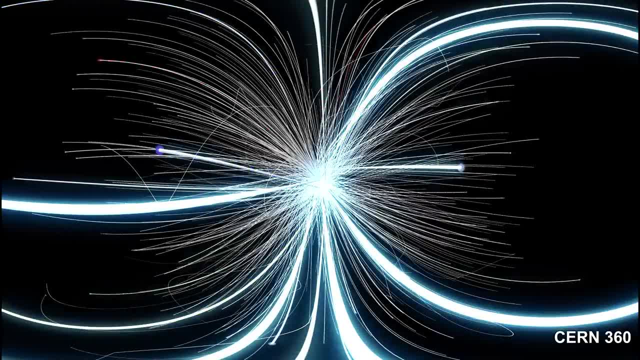 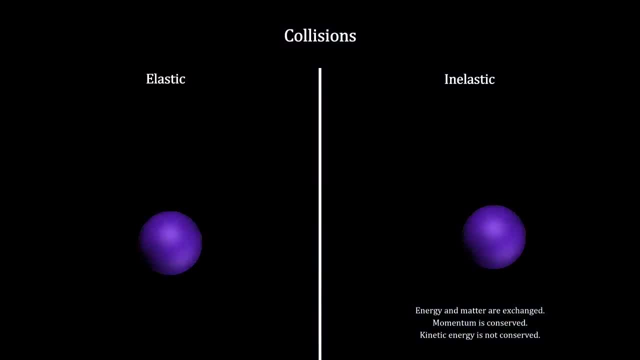 So we'll take a little time to understand what they found and the principles involved. There are two basic types of scattering. One is called inelastic scattering, where both of the colliding objects change. For example, here we have some of one object's mass. 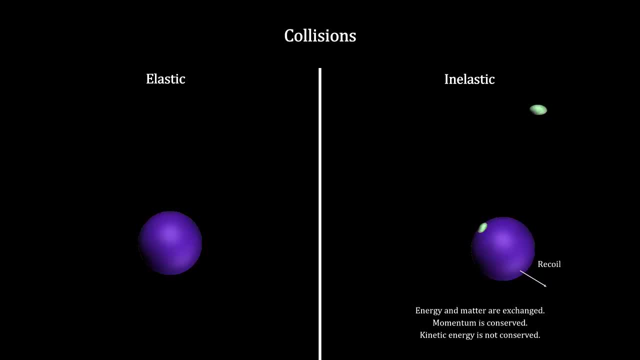 transferred to the other at the point of collision. The transfer absorbs energy, so conservation of energy doesn't hold. The other is called elastic scattering, where no parts of the participating objects are changed. Total kinetic energies are preserved or nearly preserved In both elastic and inelastic collisions. 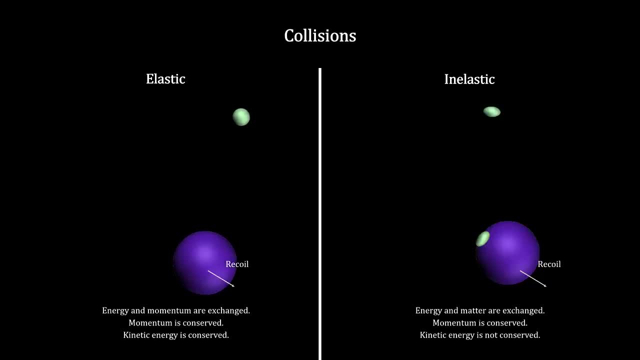 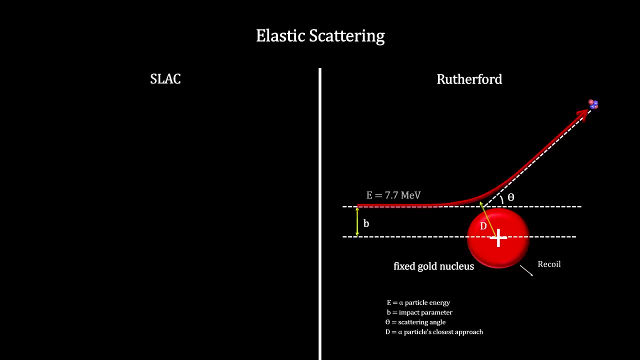 the conservation of momentum always holds true. Rutherford was examining alpha particle scattering angles off a gold atom target. to determine the size of the nucleus He had to use an alpha particle probe with fixed energy at 7.7 million electron volts. The Coulomb force was repulsive. 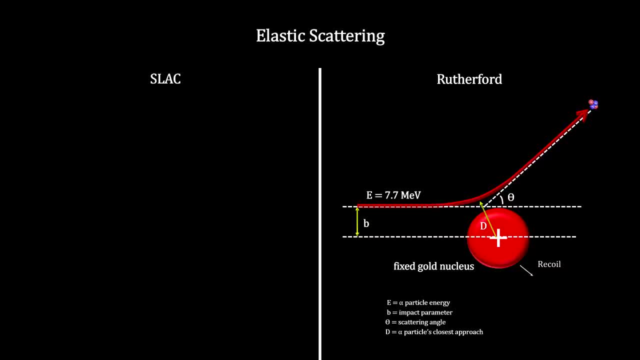 and his target nucleus was fixed in the solid gold foil, So the target recoil velocity was tiny because the entire foil had to move. The slack experiment could vary the incoming electron energy up to 17 gigaelectron volts. The Coulomb force was attractive. 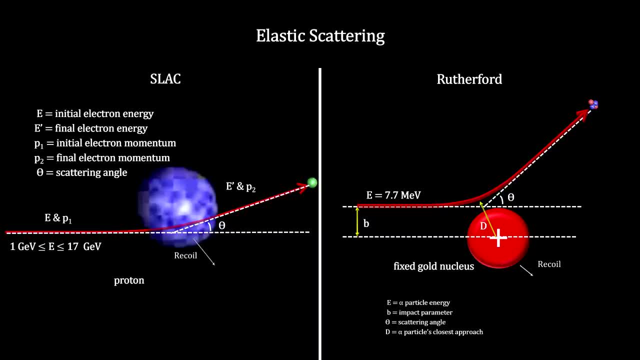 with significant target recoil when a high-velocity electron collided with a target proton. The slack experiment was designed to examine this transfer of momentum from the electron to the proton at various electron energies and scattering angles to find out if the proton's positive charge was distributed evenly. 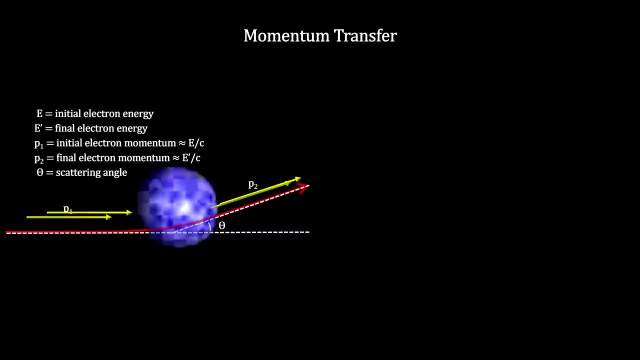 throughout its volume. The physicists controlled the incoming electron's energy and momentum and carefully measured the outgoing energy and momentum for a particular scattering angle. With that they calculated the amount of momentum lost by the electron. Given the conservation of momentum, the electron's loss 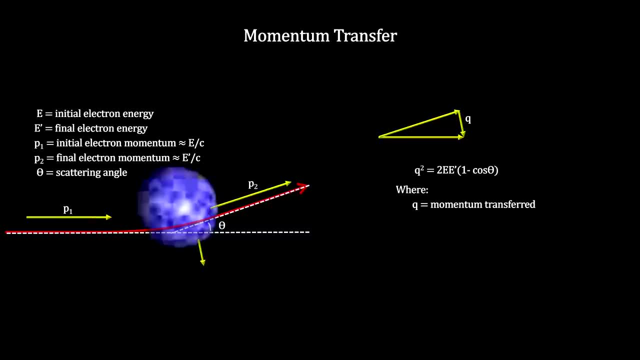 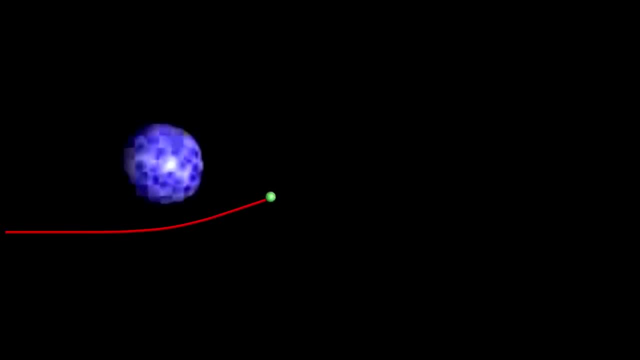 would be equal to the proton's gain. Suppose we're counting 10-degree deflections as a hit. A relatively slow-moving, low-energy electron can get a 10-degree deflection far from the center of the proton. This would make the size of the proton look large. 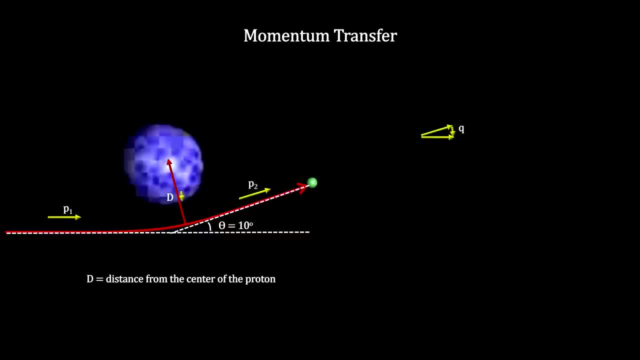 In addition, the interaction between the electron and the proton would be weak. We'd find that only a small amount of momentum would be transferred. If we increase the volume and velocity of the electron and kept its distance from the proton the same, it would not be deflected 10 degrees. 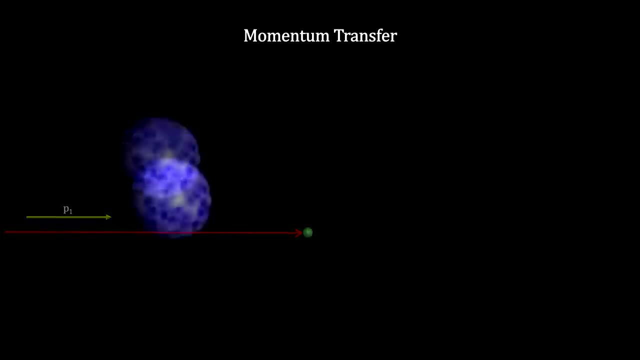 and the interaction would be considered a miss. An electron with this increased energy would have to approach closer to the proton to get deflected 10 degrees. This would have the effect of making the proton look smaller and, in addition, the momentum transfer would be greater. 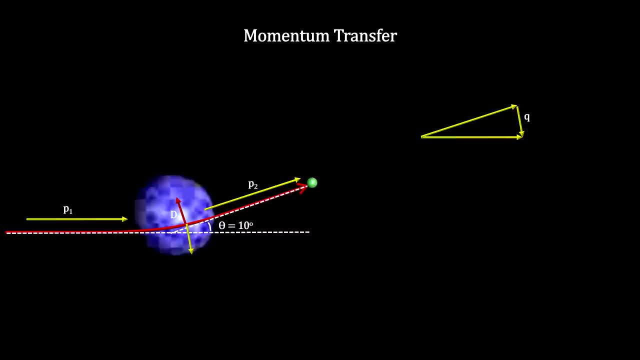 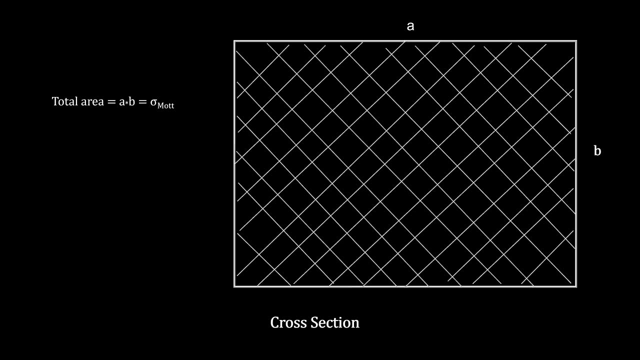 This gives rise to the concept of a cross-section. If we take a look at the total area we are shooting into and the smaller area that represents the target, we see that the probability of a hit is equal to the target size divided by the total area. You can see that as the target cross-section shrinks, the probability of a hit goes down. Of course, we only have a large number of targets in the area- the liquid hydrogen protons- so we add them together to get the total cross-section. 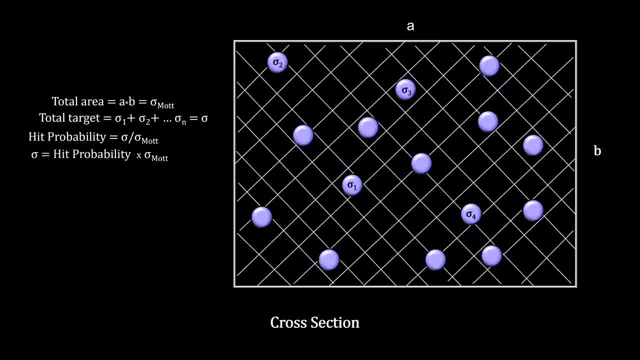 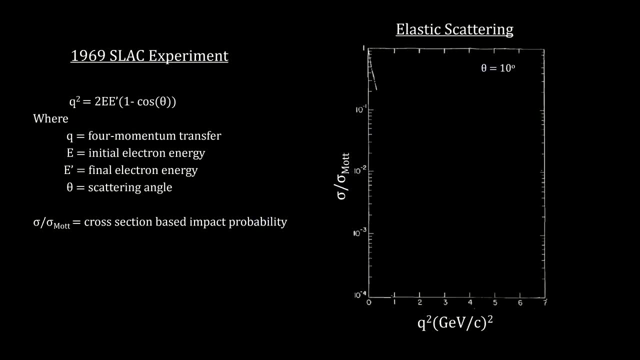 SLAC calculated the cross-section by controlling the number of incident electrons and counting the hits. Here is a graph of the interaction probabilities against the momentum transfer found by the SLAC experiment for electrons with energies below 7 GigaEV that scattered by 10 degrees. 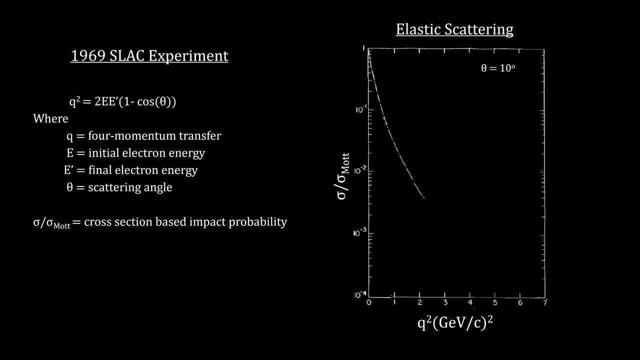 The closer to the target we get, the smaller the cross-section, decreasing the probability of a hit, while at the same time, the momentum transfer increases. with each hit that we do get, The velocity of the electrons remain the same, indicating that no energy. 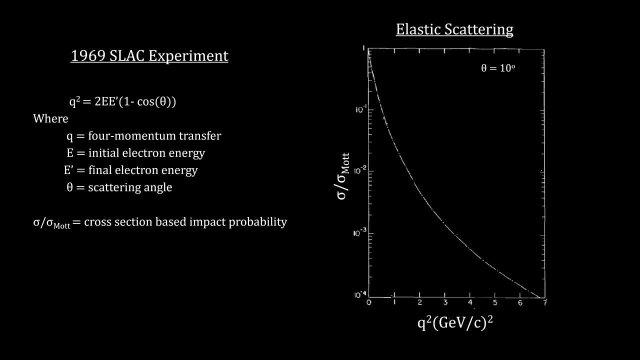 was being transferred to the proton. This is exactly what we would expect from elastic scattering, But at incoming electron energies between 7 and 17 GigaEV, this dependency changed significantly, In particular for three final proton-state energies: the momentum transfer dependence. 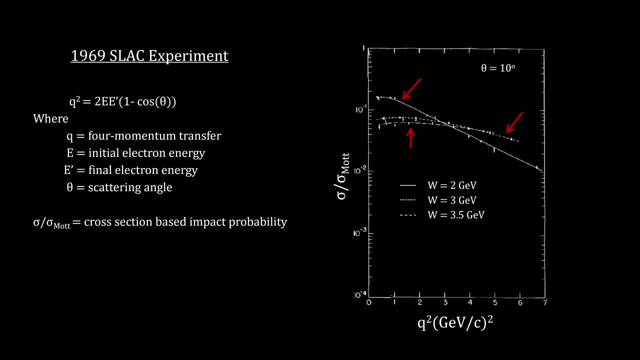 on cross-section was significantly weaker than for elastic scattering And, what's more, the protons absorbed significant amounts of energy from the colliding electrons. Physicists refer to this phenomena as resonance. To understand what's going on, we'll take a closer look. 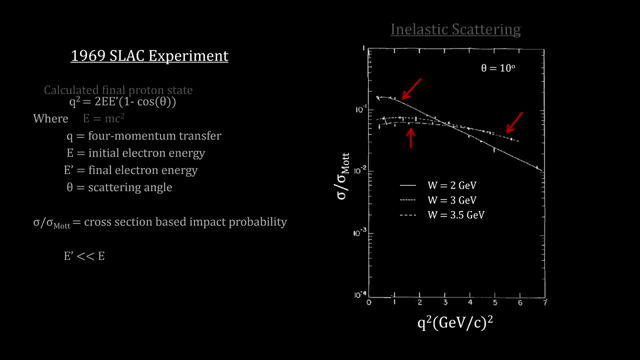 at the final proton state. You may recall that Einstein's formula for mass and energy is E equals mc squared, but this only applies to a mass at rest. For a moving particle, the energy-mass conversion includes the particle's momentum, In our case. 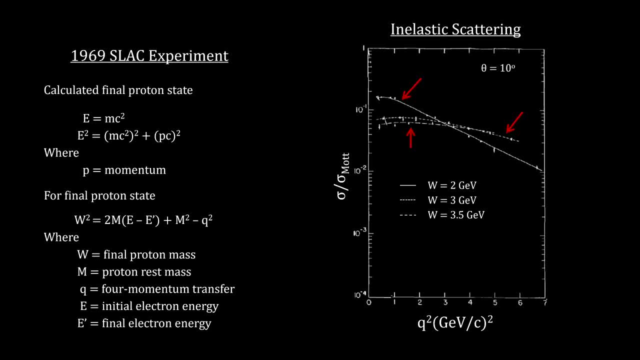 we see that the final mass of the proton goes up with an increase in energy and goes down with an increase in momentum. If you think of mass as confined energy, what is happening here is that the incoming electron's energy is being converted into increases in the mass of the proton. 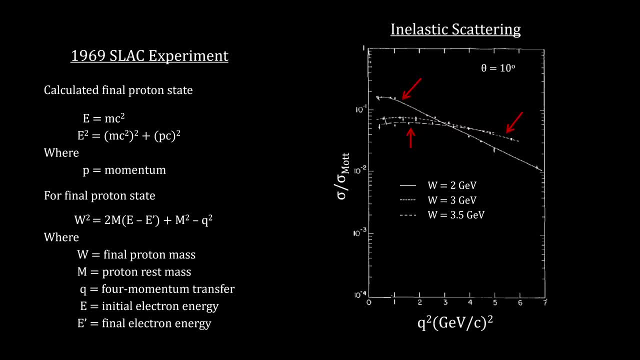 This is inelastic scattering and the three resonances indicate the proton has three internal components. Back in 1964, a quark model was proposed by Murray Gilman and George Zweig to help explain protons, neutrons and the wide variety. 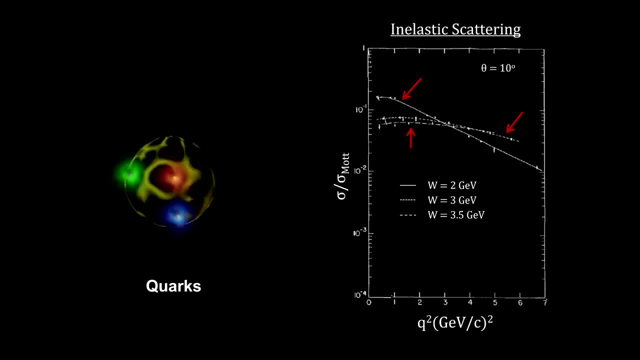 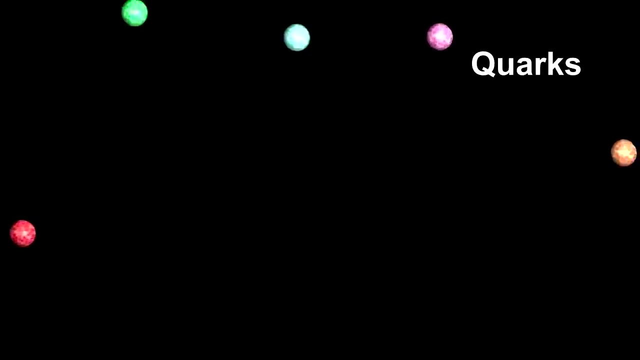 of newly discovered heavy particles like pions and kaons and others. The discovery at SLAC in 1969 that the proton has three parts constituted evidence that quarks were real. One of the key things to remember about the theory is that quarks are so strongly bound together. 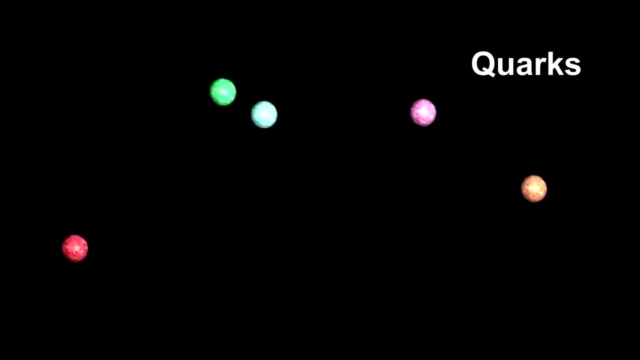 that it is impossible to study one on its own in order to determine its properties. This means that all we know about quarks is derived from the properties of the particles that bound quarks create. We call particles made of quarks hadrons, meaning heavy. 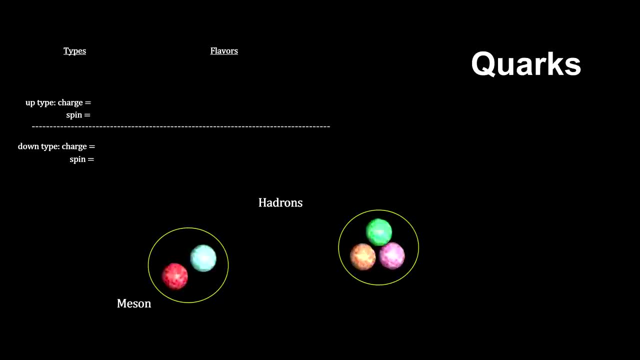 In studying hadrons we find two kinds: Those with two quarks are called mesons and those with three quarks are called baryons. All quarks have a spin of one half and the sum of quark charges needs to give us the charge of the hadron. 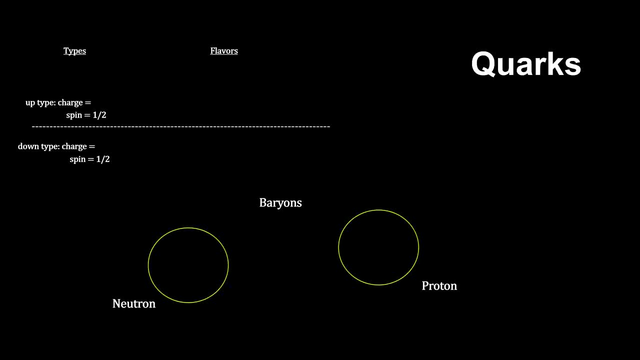 The baryons we've seen so far are the proton and the neutron. Quark theory has it that there are two flavors of quarks that make up these baryons, called the up quark and down quark. Protons have two up quarks. 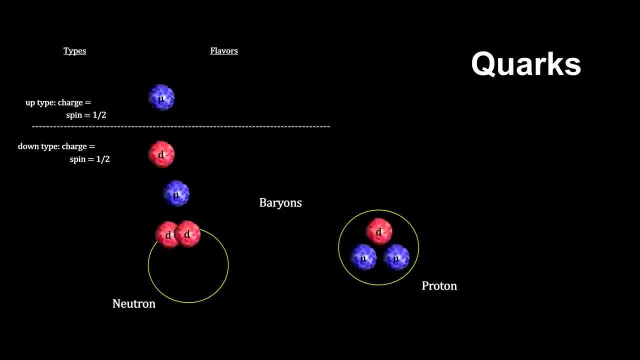 with one down quark and the neutron has one up quark and two down quarks. In order to get the correct charge of the proton and the neutron, the up quark must have a positive charge, that is, two-thirds the charge of an electron. 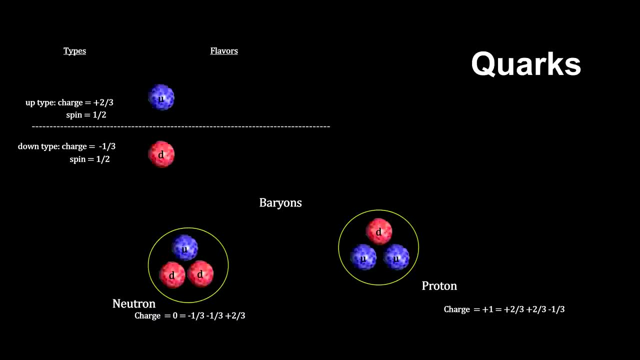 The down quark must have a negative charge, that is, one-third the charge of an electron. The down quark must also have a little more mass than the up quark for the neutron to have a little more mass than the proton. Note that the sum of the quark masses. 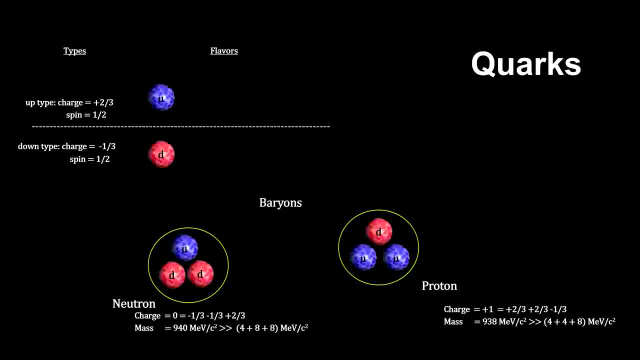 falls far short. This indicates that there is a lot more going on inside the proton than we've seen so far. The up and down quarks are the lightest and most stable quarks, and all other quarks will decay into these two over time. 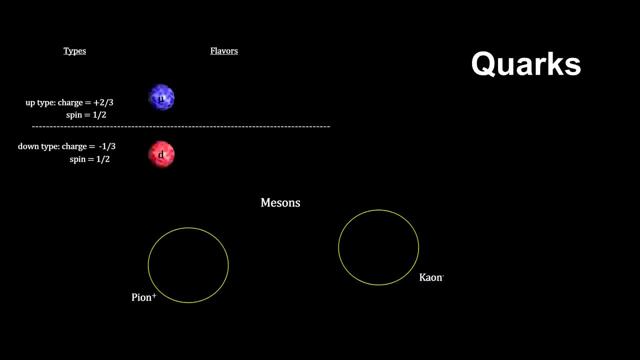 The two mesons we've seen are the pion and the kaon. The positively charged pion has an up quark and an anti-quark. The up quark has a positive charge and an anti-down quark, The negatively charged kaon. 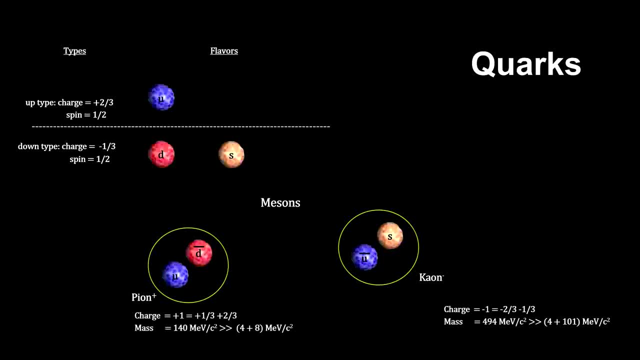 contains an anti-up quark and a third kind of quark called the strange quark. It was needed to explain the length of time it took the kaon to decay. In addition to the up down and strange quarks, we have discovered the charm. 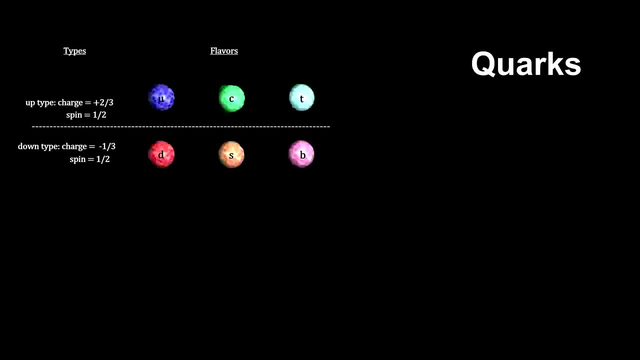 top and bottom quarks for a total of six. One of the key rules seems to be that they can only combine in combinations of two or three as long as the sum total of charge always equals the charge of an electron or a proton or zero. 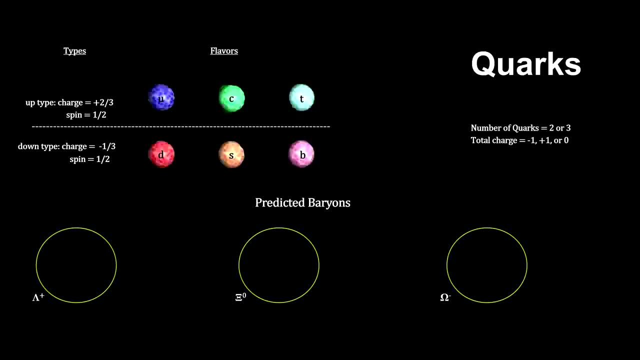 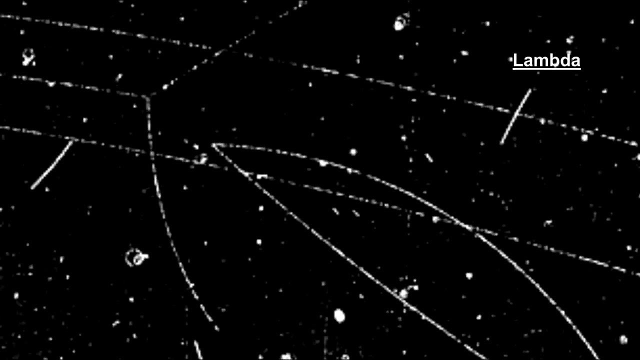 So armed with quarks. physicists intensified their search for some of the three quark particles predicted by Gilman and Zweig's theory: the lambda, psi and omega baryons. In 1947, the lambda particle was discovered. Here we see a V shape. 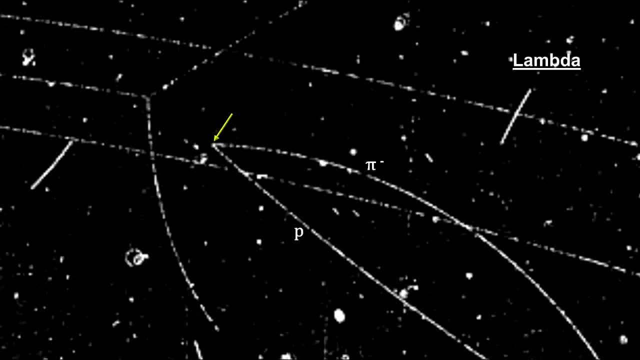 with the creation of a pion and a proton. It was the proton that told us the decaying neutral particle lambda must have had three quarks. The particle was expected to live for about 10 to the minus 23 seconds, but actually survived. 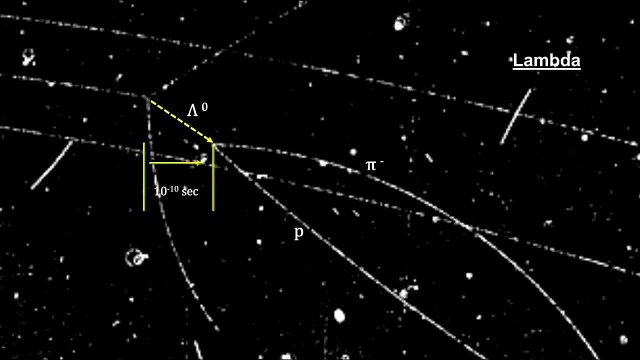 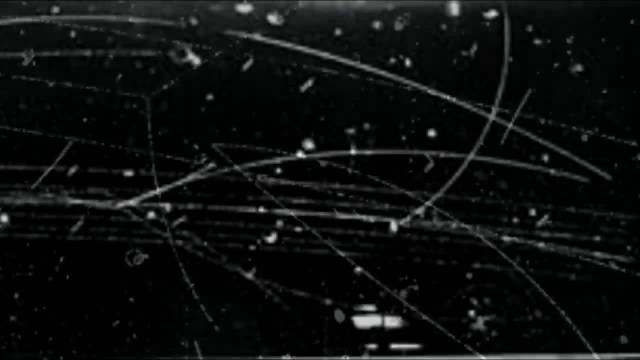 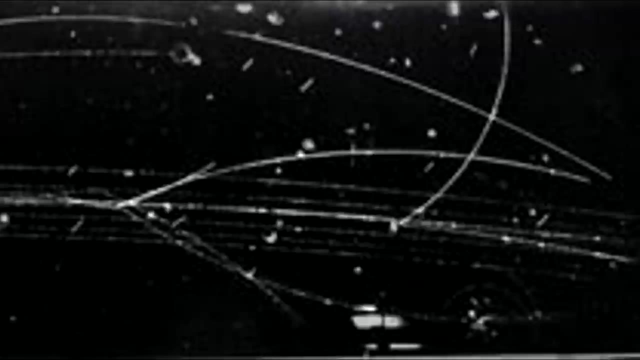 for 10 to the minus 10 seconds. The property that caused it to live so long was dubbed strangeness and led to the discovery of the strange quark. In 1964, the psi baryon was discovered at the Brookhaven National Laboratory. 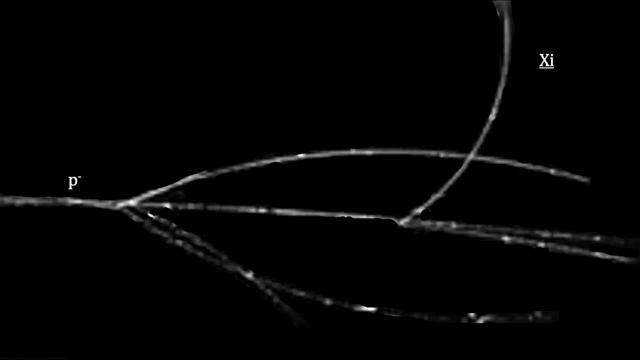 Anti-protons arrived from the left. One of these anti-protons collides with a hydrogen nucleus, a proton, resulting in mutual annihilation. The mass of the proton and the mass plus kinetic energy of the anti-proton give birth to two heavy particles. 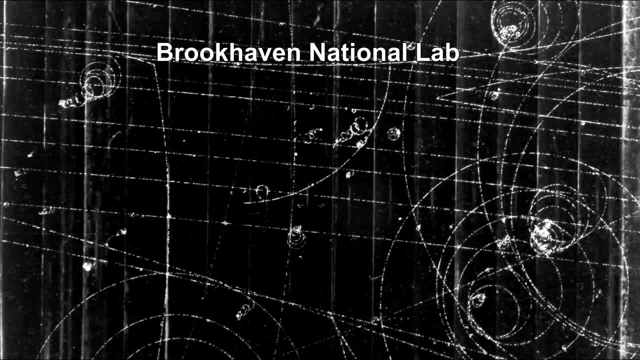 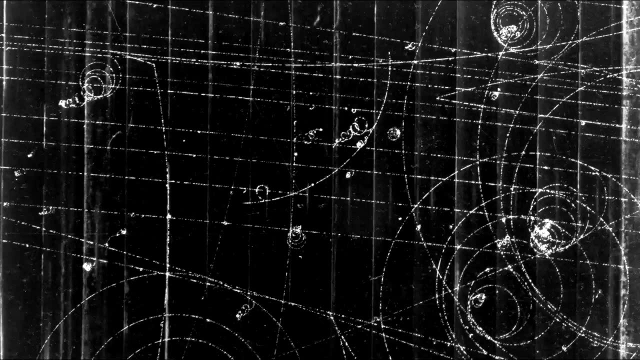 a negative psi and its anti-particle. Also in 1964, at the Brookhaven National Laboratory, the omega particle was discovered. This is one of the most famous bubble chamber pictures of all. It shows the discovery of this long predicted particle. 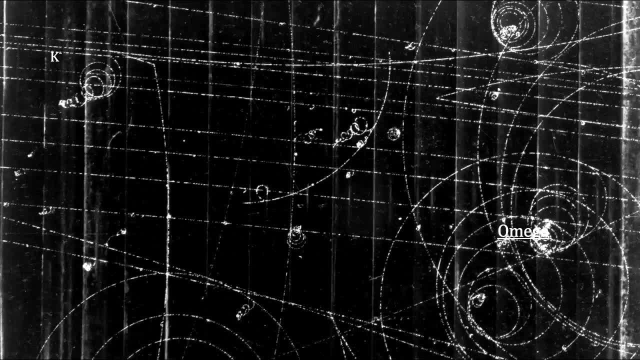 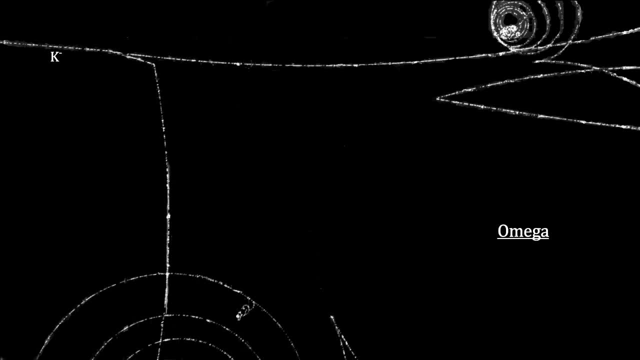 In this photograph you can see it entering the chamber on the left To help see the omega particle. I'll remove all but the tracks associated with the omega event and work backwards from the V on the right. that creates a pion and a proton. 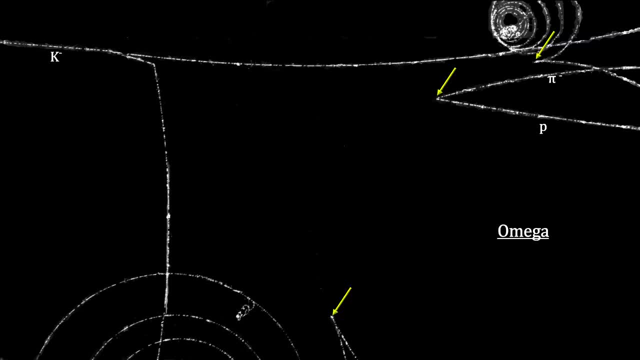 This is the trademark decay signature for the lambda particle. We also see Vs in the upper right and in the lower middle where positron and electron pairs form. If we draw lines back to where the lambda particle and the two gamma rays cross, we see that a neutral particle. 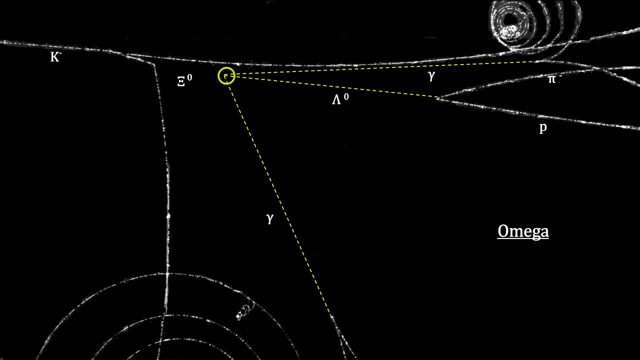 decayed into the neutral lambda and the two gamma rays. This is the decay signature for the neutral psi particle. We can now draw the path of the psi particle back to the kink, where another particle was decayed into the neutral psi and a pion. 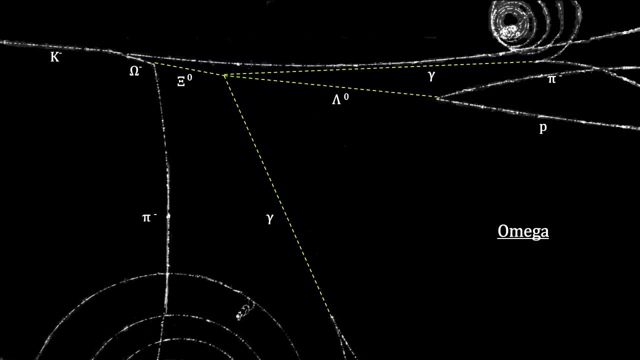 This fit the expected properties of the omega particle. that's made up of three strange quarks Tracing the path of the omega particle back to the kink. in the path of the kaon we can see the decay that created the omega particle and measure the length of time. 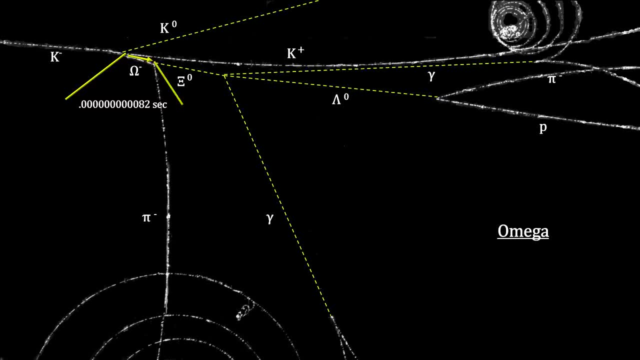 the omega particle existed. It has a very short life of 82 trillionths of a second. The physicist working on analyzing this photograph was so excited about his find that he invited the director of the Brookhaven Laboratory in the middle of the night to give him the news. 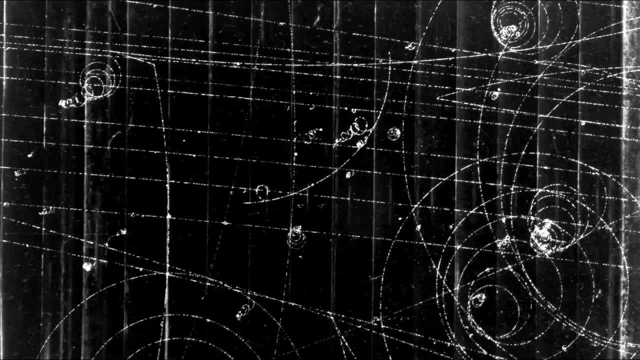 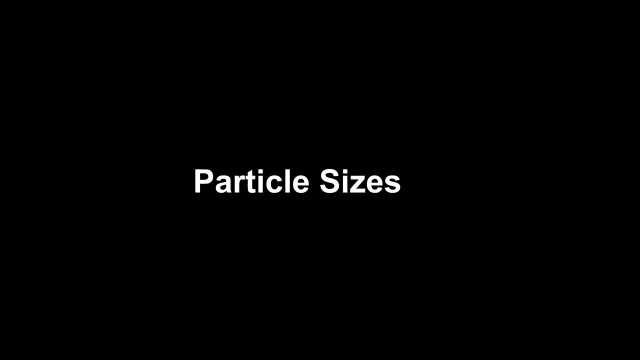 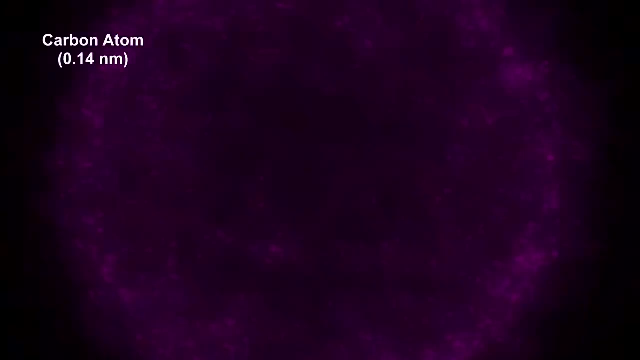 As with other predictions of previously unobserved particles, this discovery gave a tremendous boost to quark theory. Now's a good time to review the particle sizes we've seen so far. In our first segment, we used an electron microscope with a diameter of 0.14 nanometers. 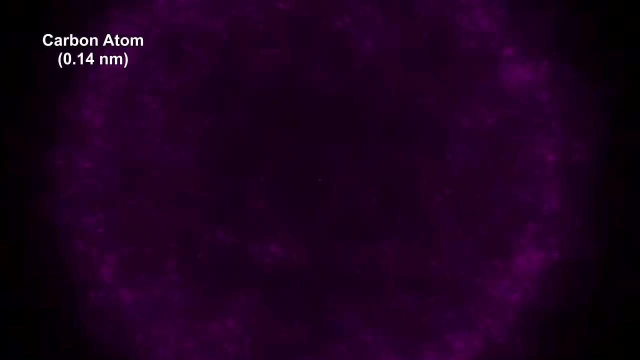 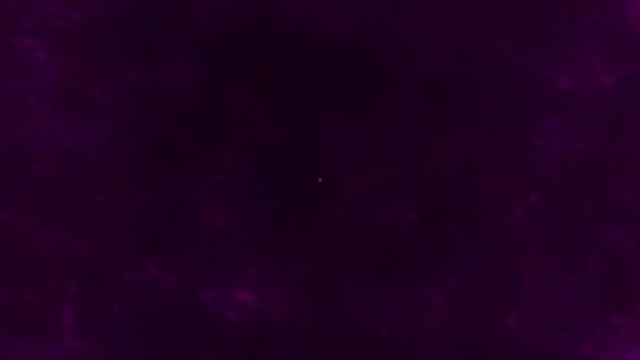 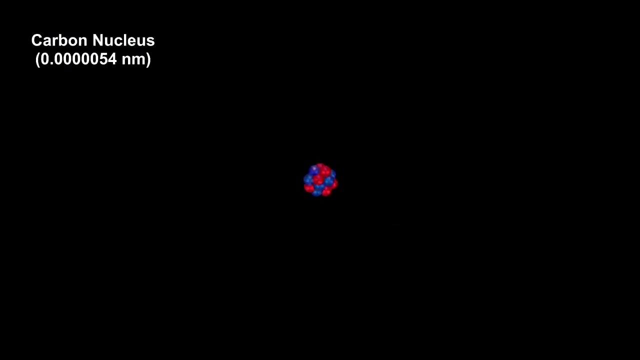 That's a million times smaller than the width of a human hair. In our second segment, we probed the atom with alpha particles and found that the nucleus was very small compared to the atom. Here we have the carbon nucleus at around 26,000 times smaller. 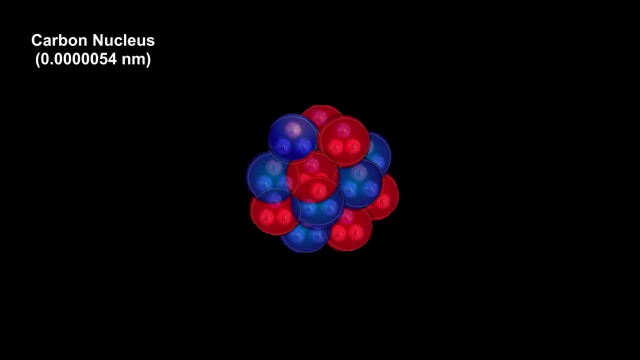 than the carbon atom. The simplest nucleus is hydrogen's. It's just a proton. At this level, the nanometer is way too large, So we'll move to femtometers instead. There are a million femtometers in one nanometer. 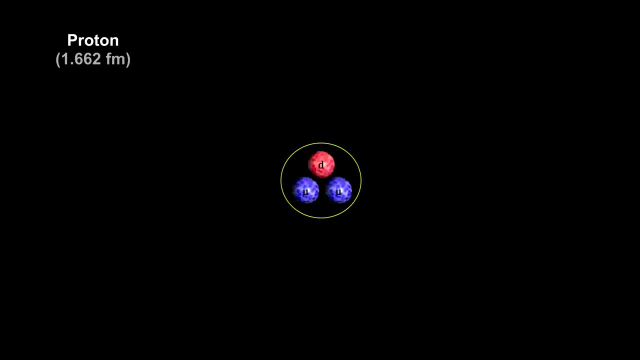 Modern experiments have produced excellent results and show that the diameter of a proton is 1.662 femtometers. In this segment, we probe the proton with high velocity electrons and found that it contained three quarks Powerful accelerators and hadron colliders. 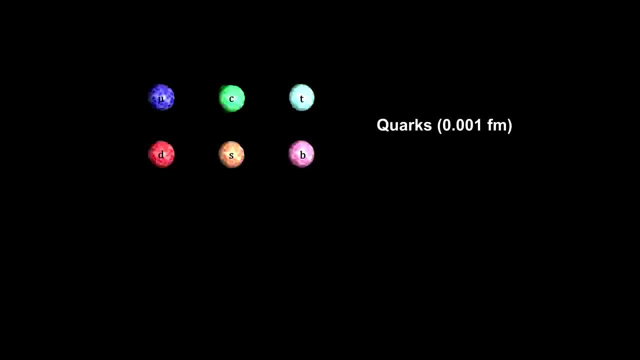 have put the upper limit on the diameter of the cross section of a quark at 0.001 femtometers. That's 1,760 times smaller than a proton and 140 million times smaller than a carbon atom. This is also the upper limit. 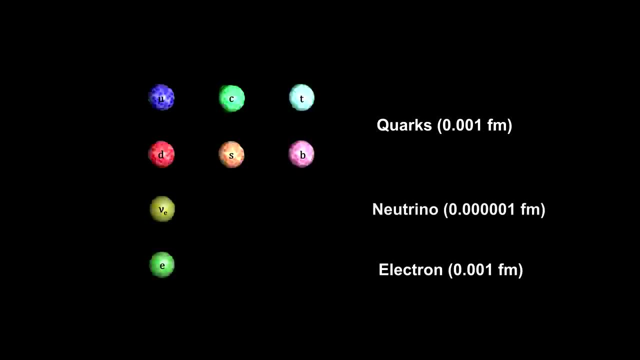 for the cross section of an electron. The neutrino is the smallest elementary particle, with a cross section that is a thousand times smaller than an electron or quark. That makes it 140,000 trillion times smaller than the diameter of a human hair. 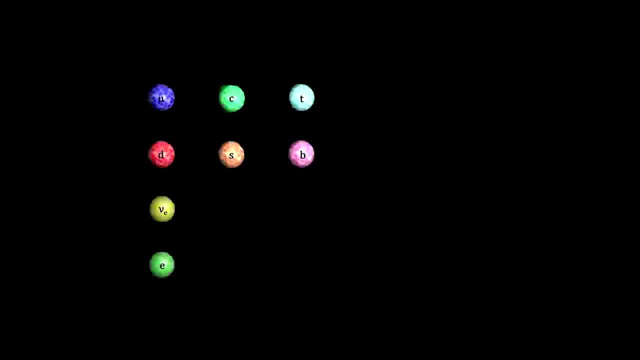 When confronted with a vast number of observations, the first step to understanding is categorization. We try to find the similarities and differences between things. When it comes to elementary particles, we have already made some distinctions. We have the small light particles like the electron and the neutrino. 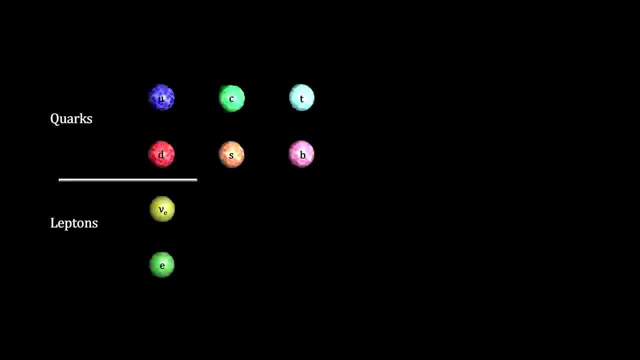 called leptons, And we have the quarks that make up the heavy particles, like protons and neutrons, called hadrons. Everything we see around us is made of these three particles: the quark and the down quark, A particle's spin. 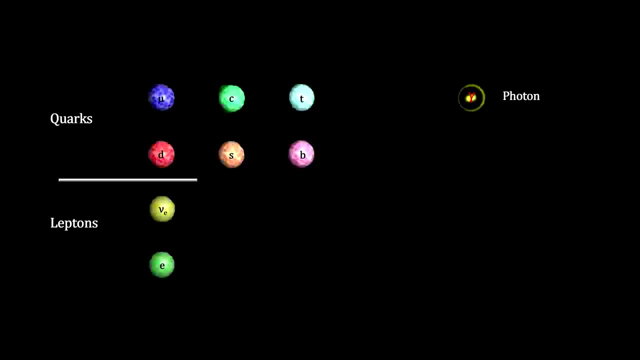 is another key distinction that helps us categorize all these particles. You'll recall that electrons and quarks have spin one half and therefore follow Pauli's exclusion principle. Photons have spin one and do not follow the exclusion principle. The statistics that describe: 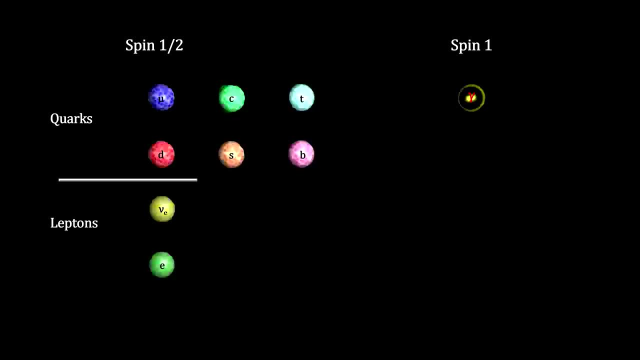 spin one half particle behavior was developed by Enrico Fermi and Paul Dirac. They are called fermions after Mr Fermi. The statistics that describe spin one particle behavior in large groups was developed by Satyendra Nath Bose and Albert Einstein.